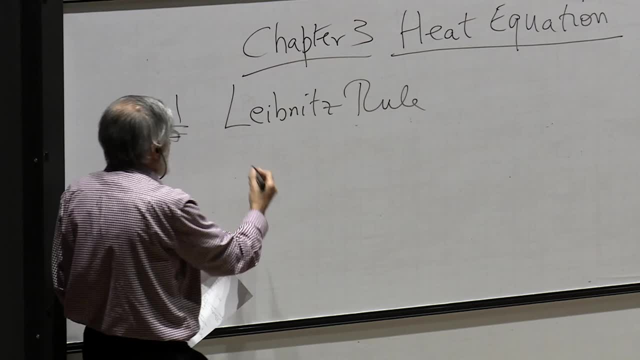 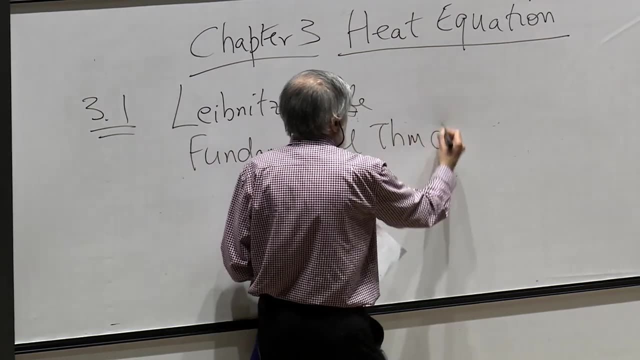 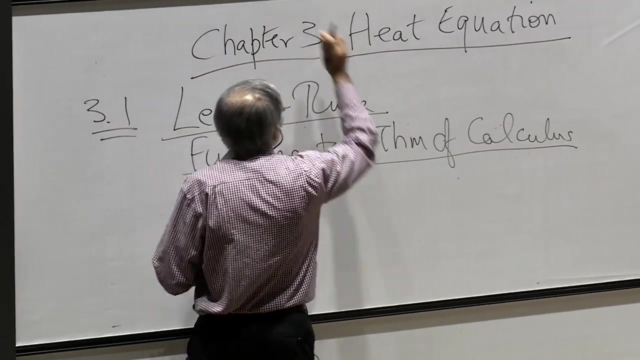 swapping and integration, And in the notes we've got the Leibniz rule about integration, swapping and integration, integral and derivative- and we've got the fundamental theorem of calculus, which is what we did. we've already covered those, okay, so we can go. 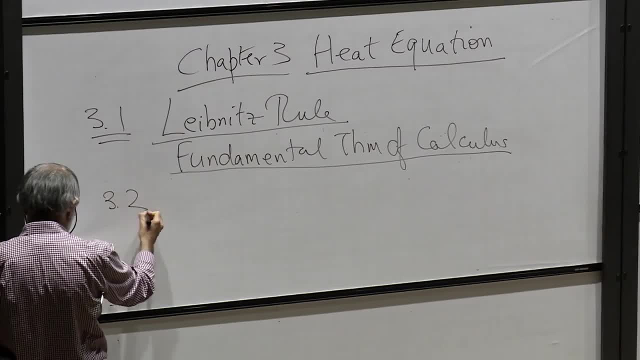 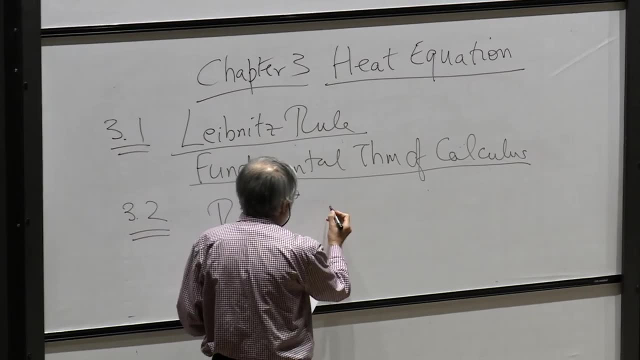 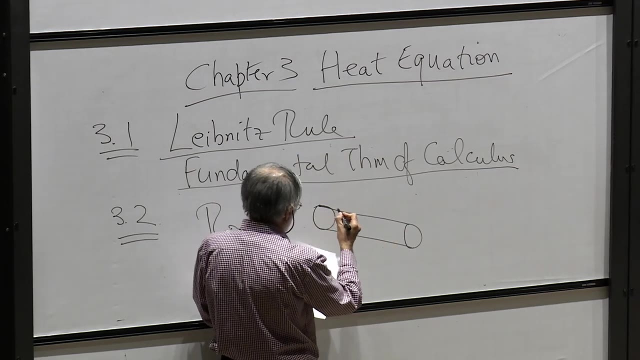 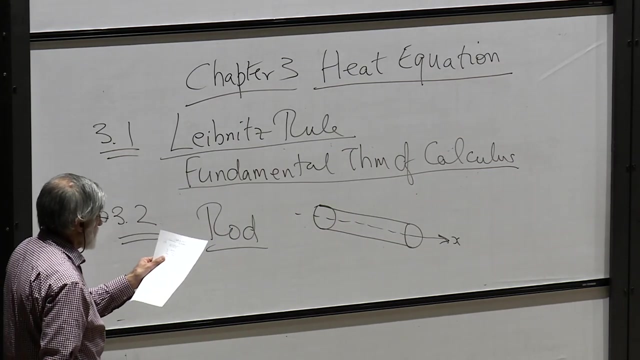 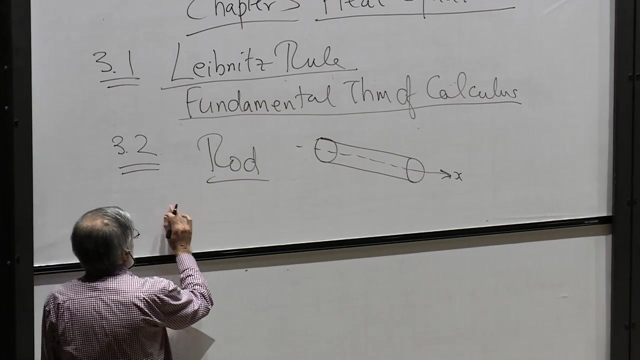 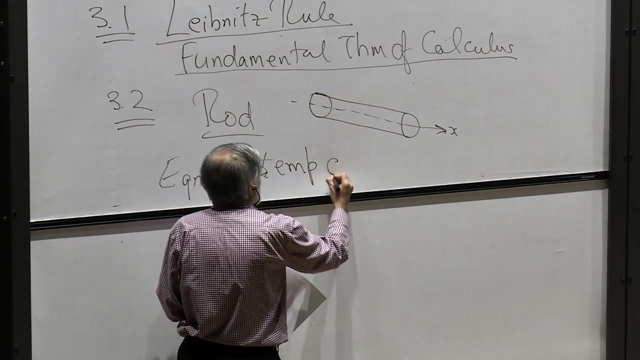 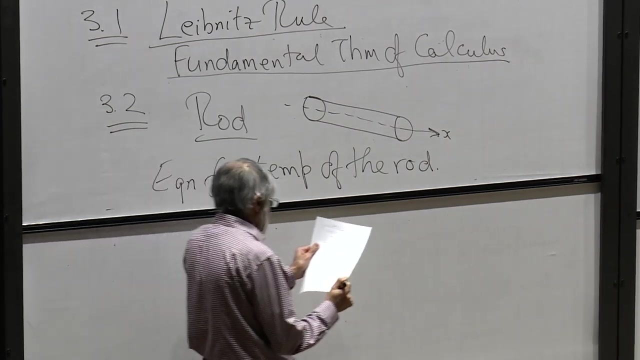 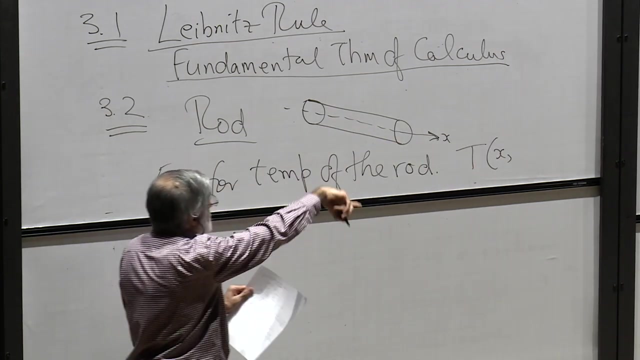 straight now to three, point two. so suppose we have a rod and let's suppose the rod looks like this, where this is X, X direction. okay, and what we want to do is you want to find out equation for the temperature of the rod. so the temperature will be T and it'll depend on X. we're just 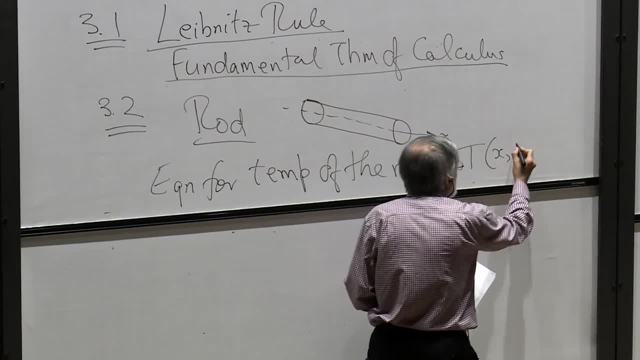 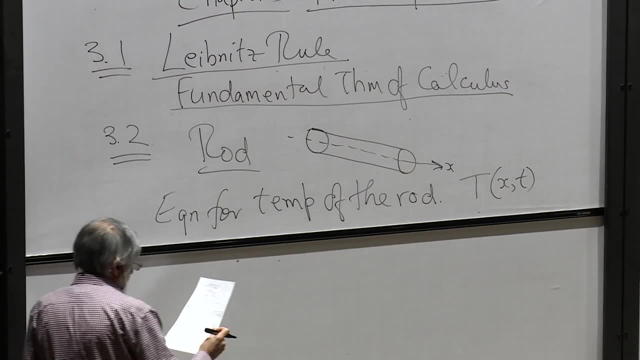 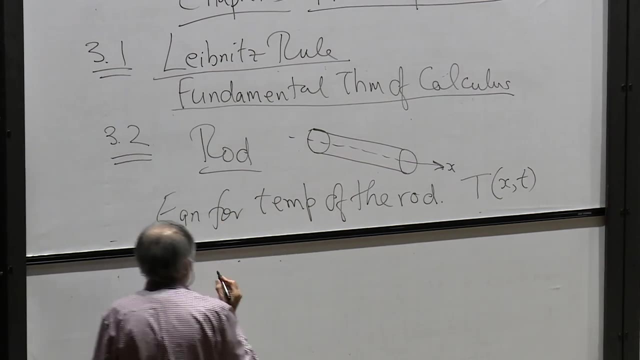 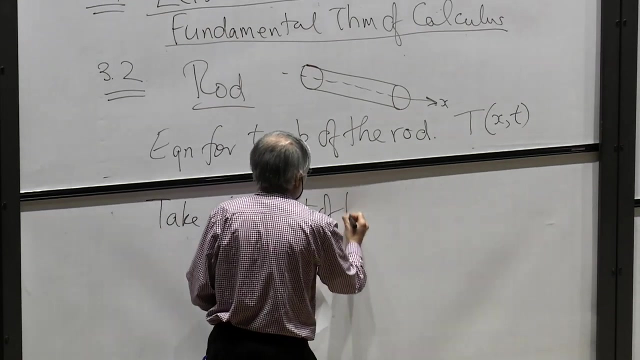 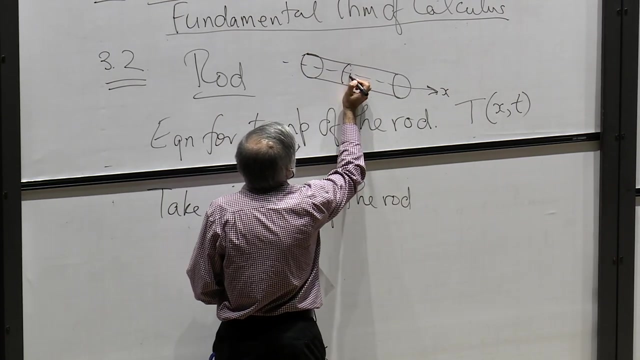 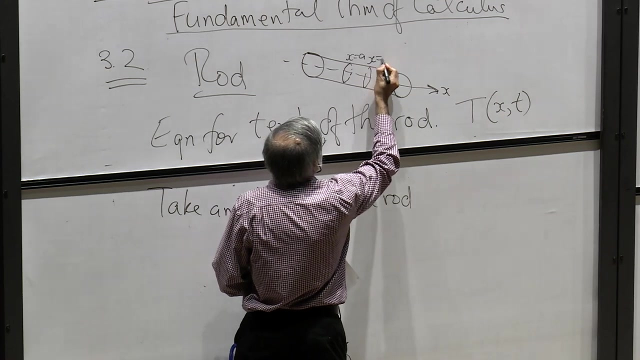 essentially assuming this is a one-dimensional thing- and little t, which is time, right. so what we do then is we use conservation law. so we take a little element, the temperature. we take a little element, element, take an element of the rod, so a little element like this, that's: x equals, a x equals. 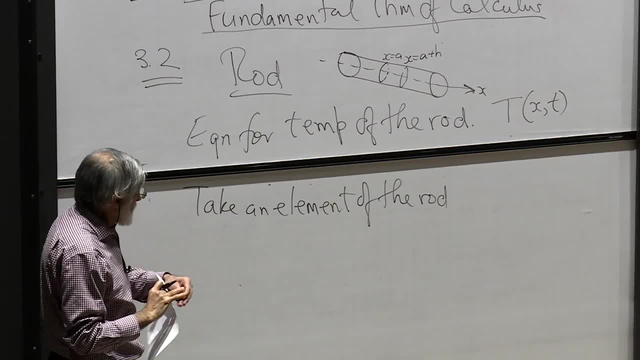 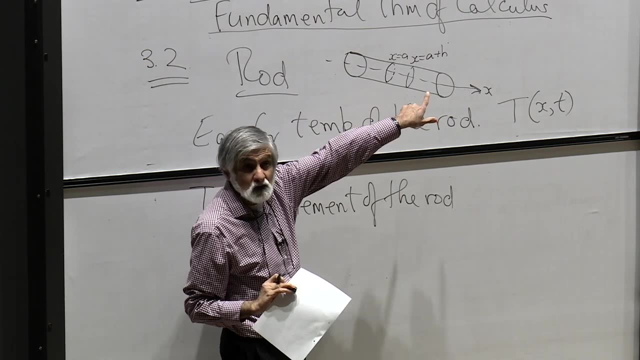 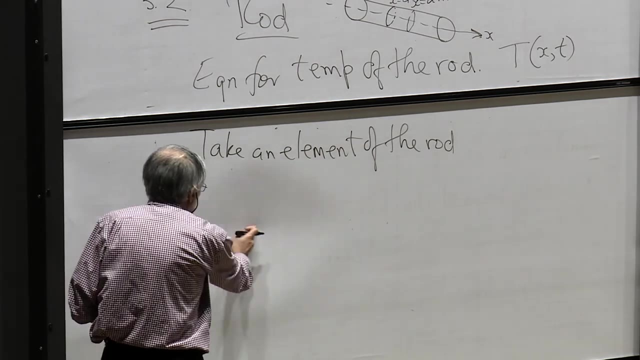 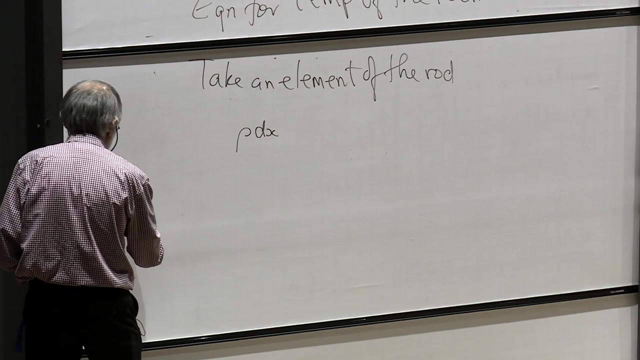 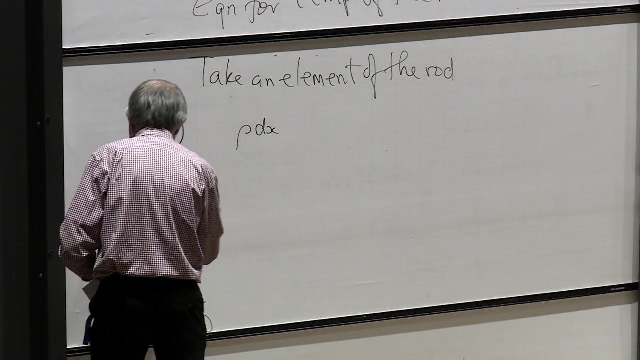 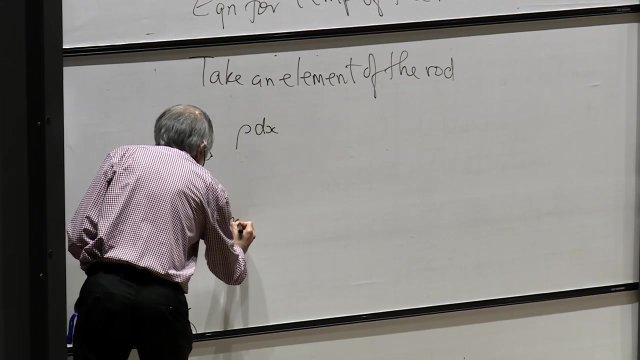 a plus h. and now what we're going to ask is: how does the heat change in this element? So if we have that element, then what we have is rho times delta x, where rho is density and a is cross-sectional area. so it's probably better not to write this and wait until I've 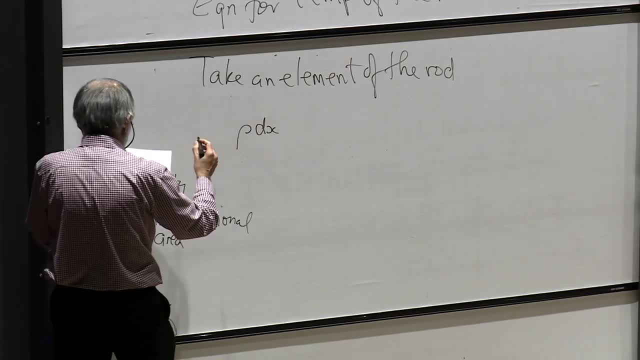 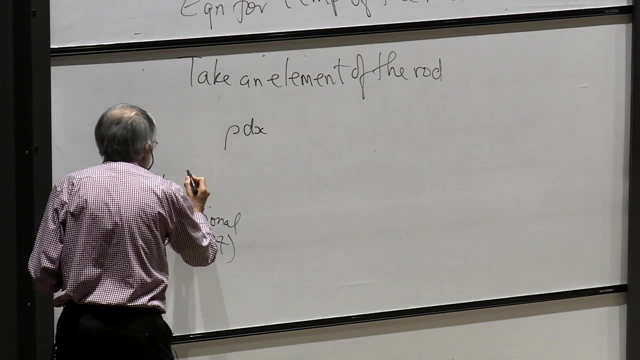 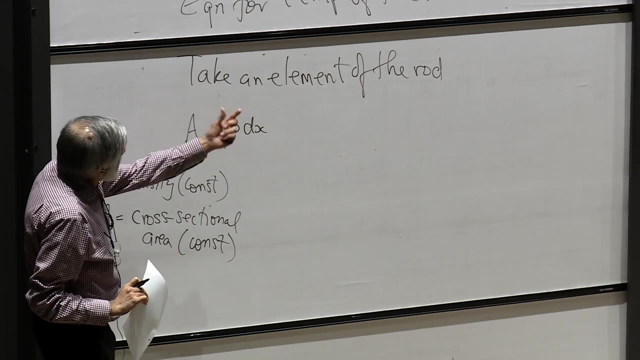 written it all down, and then write it okay and put the a and, which we assume is constant. it's constant and we're assuming the density is constant, right? so if you think about it, if you take now a little tiny, 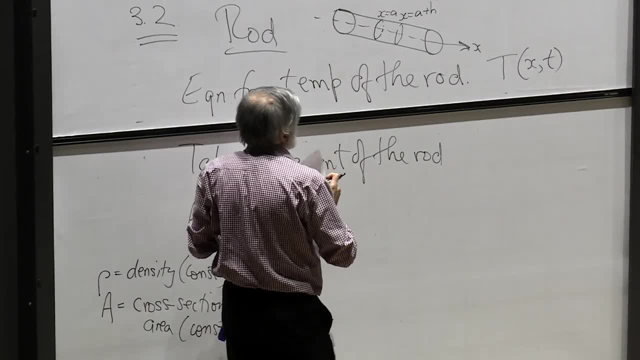 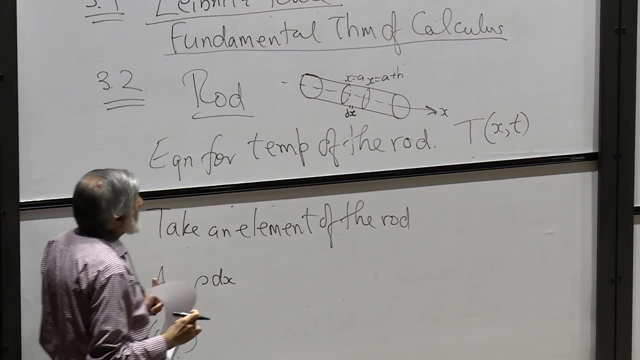 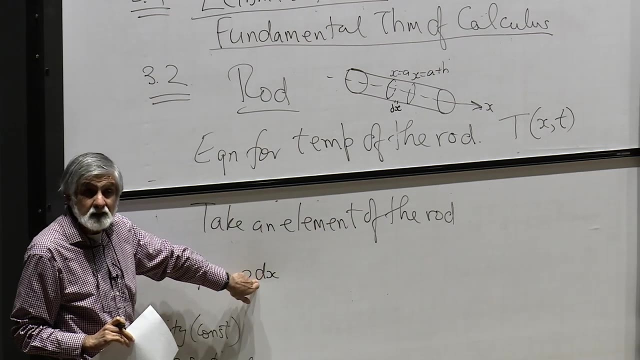 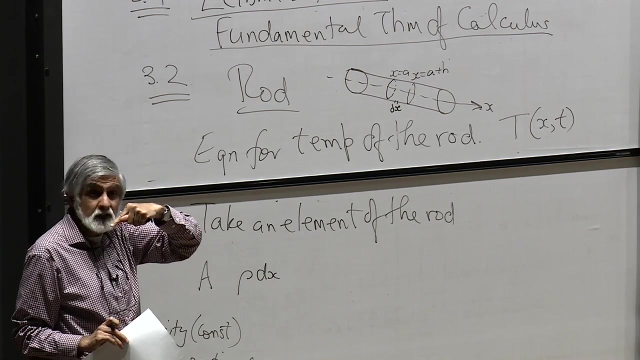 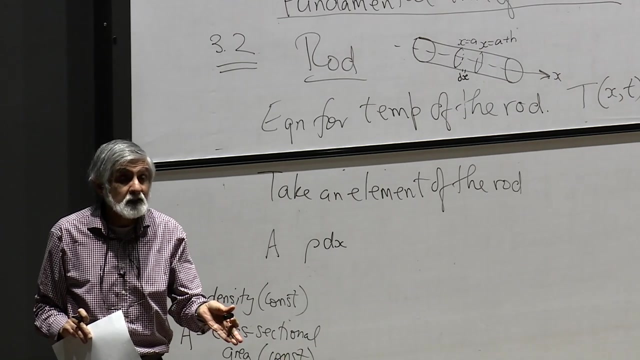 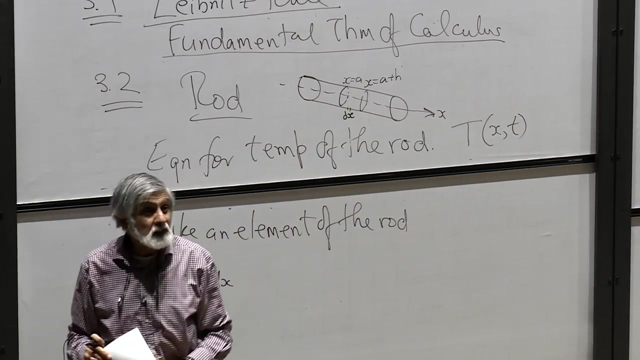 delta x in here, then the volume of that will be a times delta x, because it's a disc with circular area, a height dx. so volume is a times delta x multiply by rho give and that gives you the mass. okay, so that's the mass of this little volume and the that little. 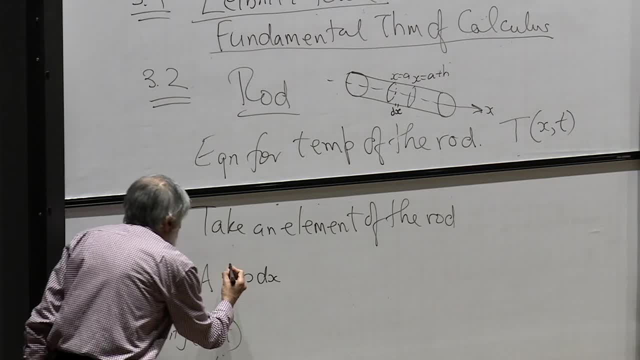 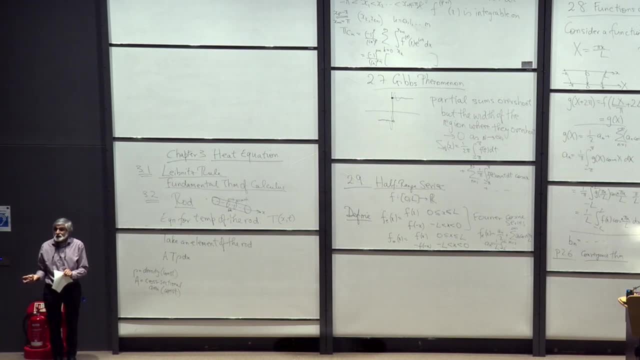 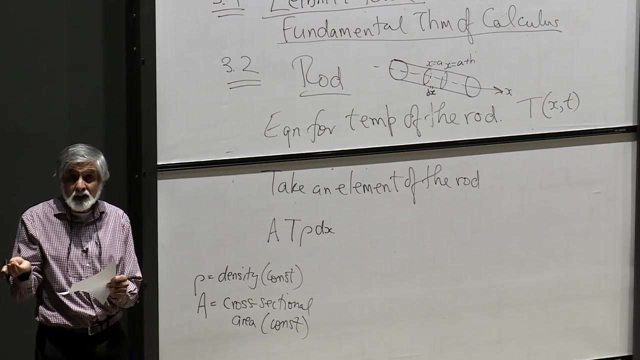 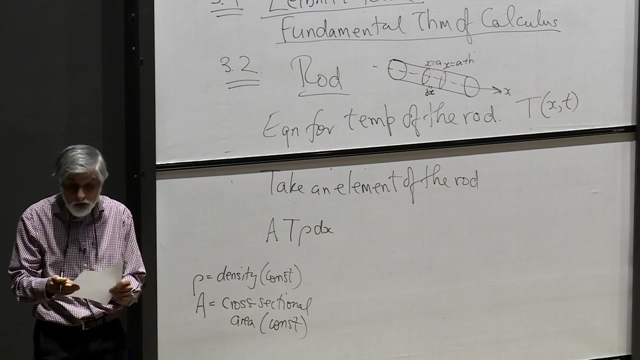 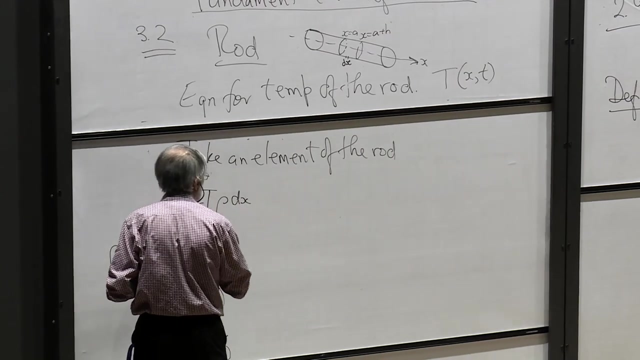 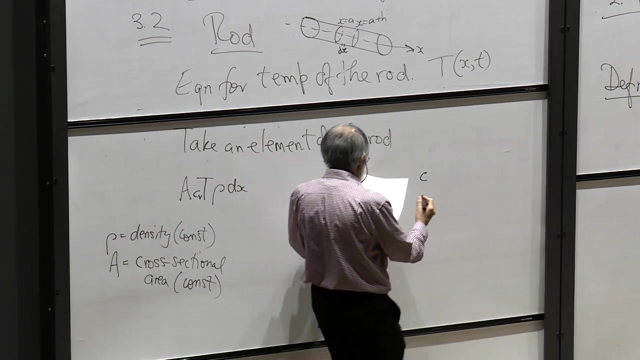 volume, if delta x is very small, will have exposed to temperature t. and then we have to do is you have to say: okay, how does that temperature t convert into heat? Okay, So heat is related to temperature, so there must be a constant of conversion and that constant is called C, and so C or Cv is called in the notes Cv, that's called the Pacific Heat Capacity. 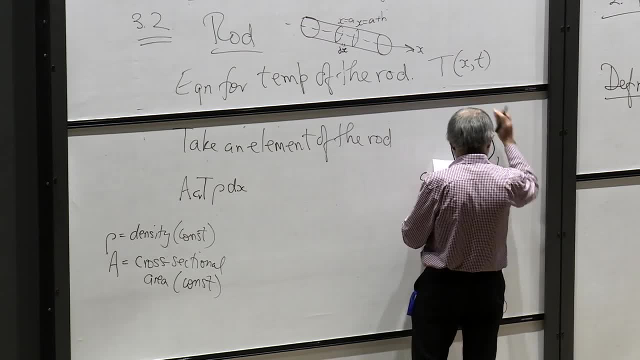 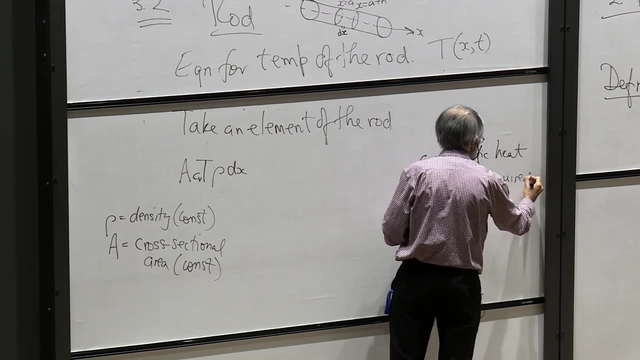 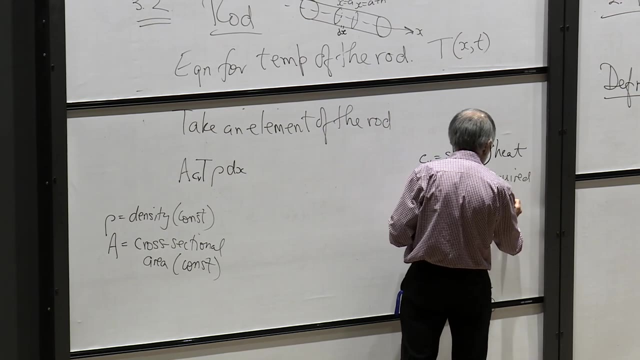 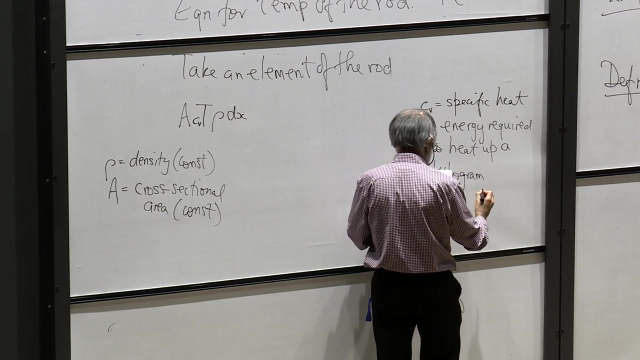 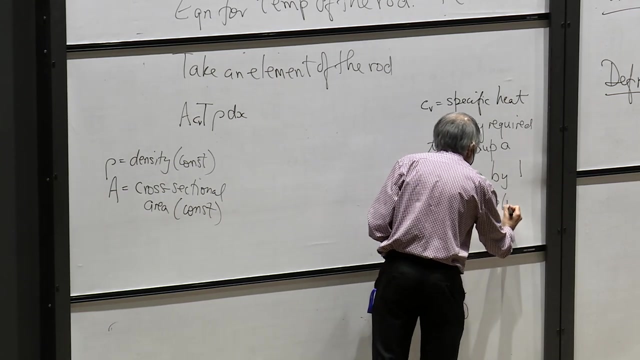 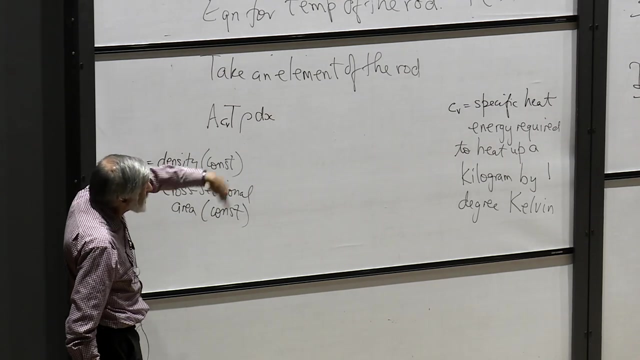 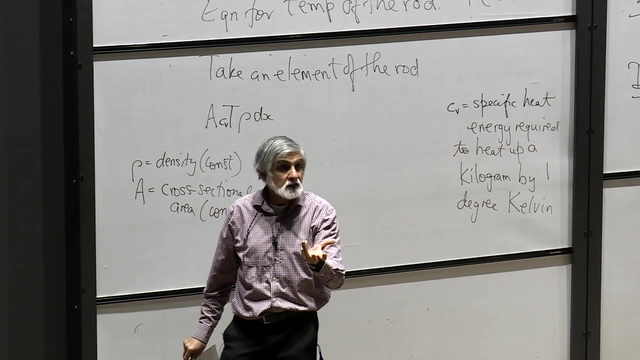 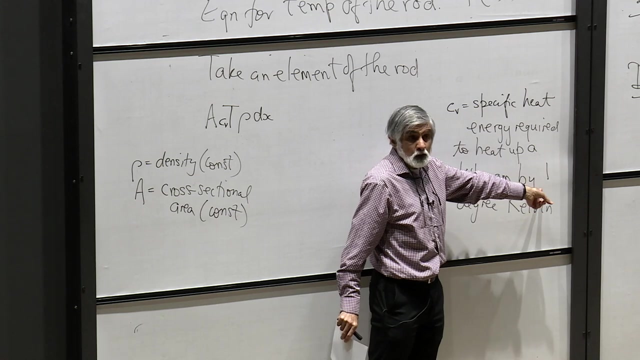 which is the energy required to heat up a kilogram by one degree Kelvin. Okay, so if that's the energy. so basically, that's the energy that a material has if it's one kilogram and it's got one temperature of one degree Kelvin. 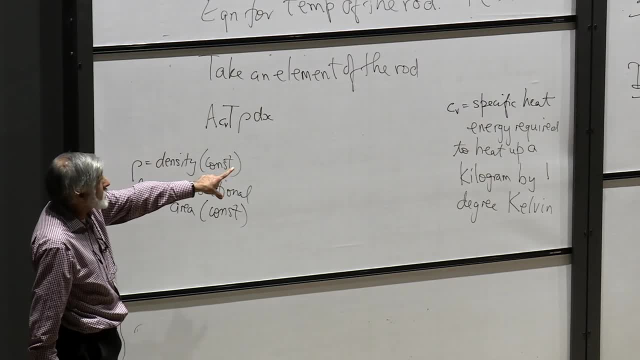 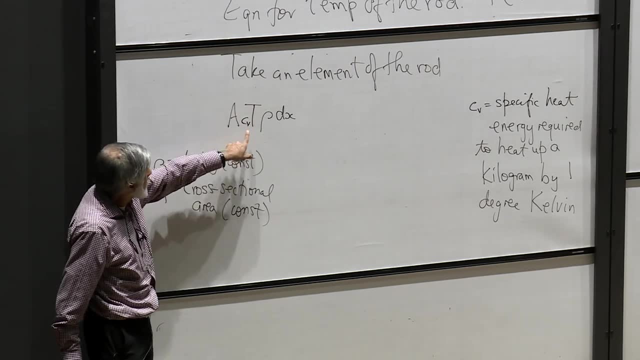 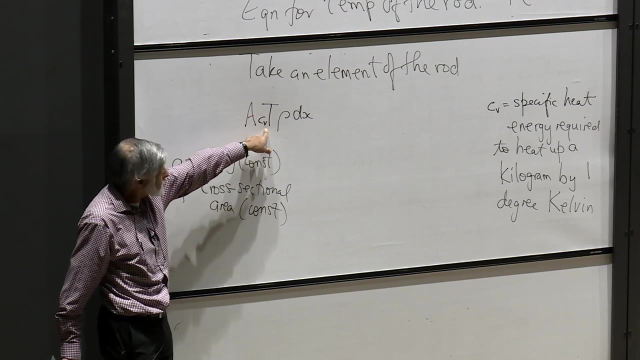 Okay, so if that's the energy For one degree Kelvin, if we measure T in Kelvins, Cv times T will be the energy for T. as long as big T is in Kelvins That will be for a kilogram. but we don't have a kilogram. 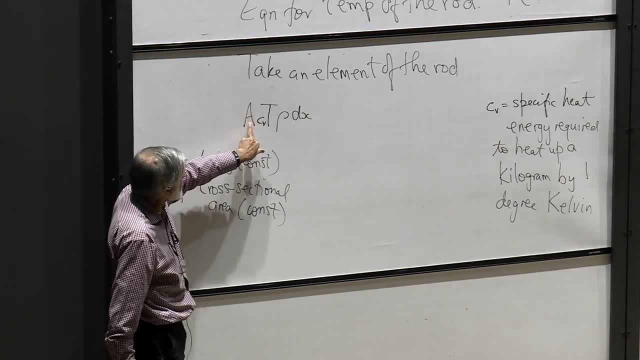 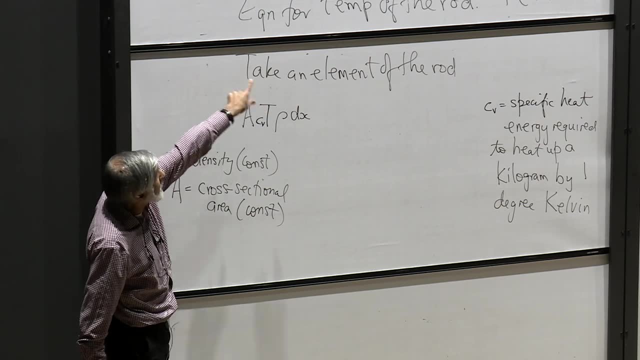 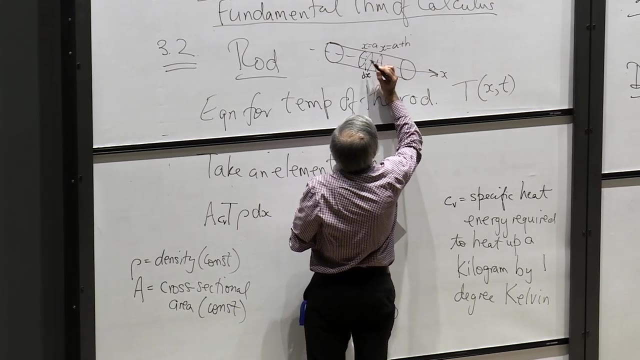 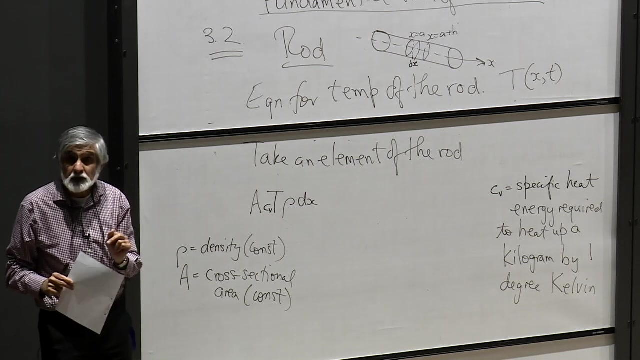 What's the mass we have? The mass we have is A rho dx, So this is the heat energy within the little sort of element delta x. And now, you see, crucially here is that we have to make sure that all these have the right units. 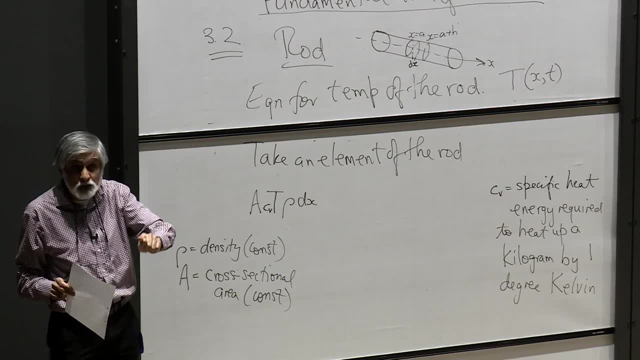 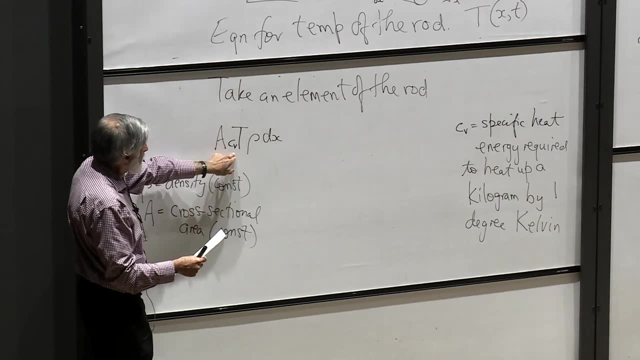 And I'm not writing down the units because the units are listed in the notes, so there's no point in me just repeating the units. Okay, there's a nice table in the notes that has all these units. So this is the amount of heat energy. 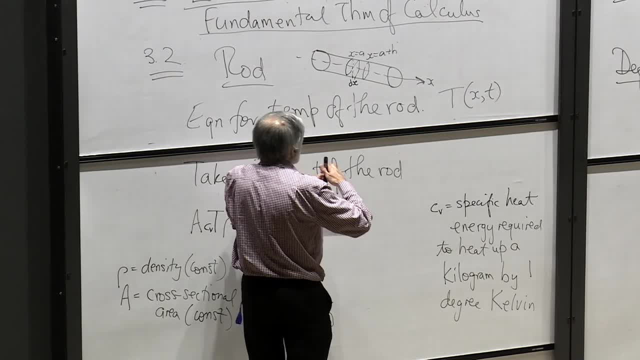 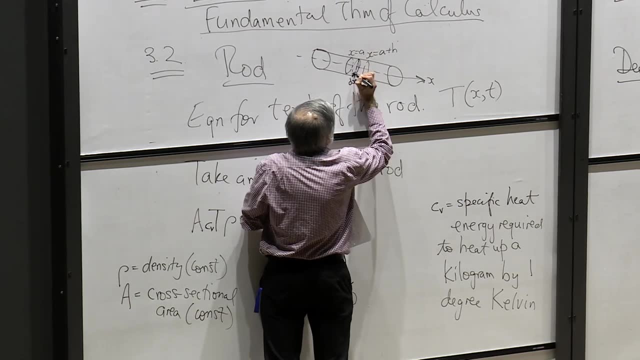 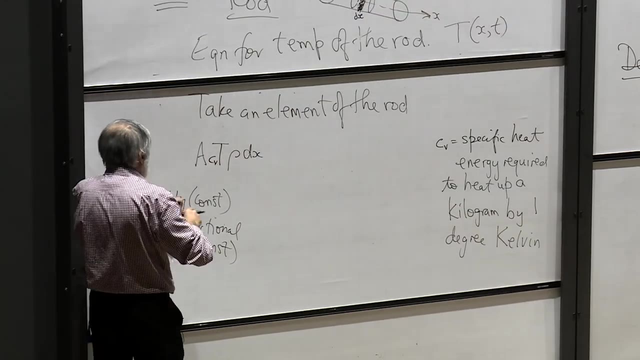 in this little region. So I did that wrong. That should be like that. and then there's another one like that. So that's in this little sort of region, like that. So now, obviously, what we need to do is we need to integrate that. 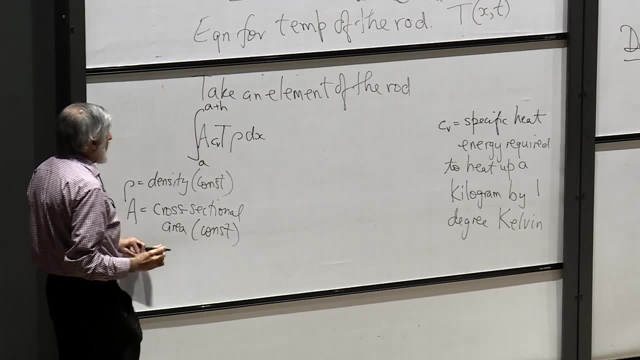 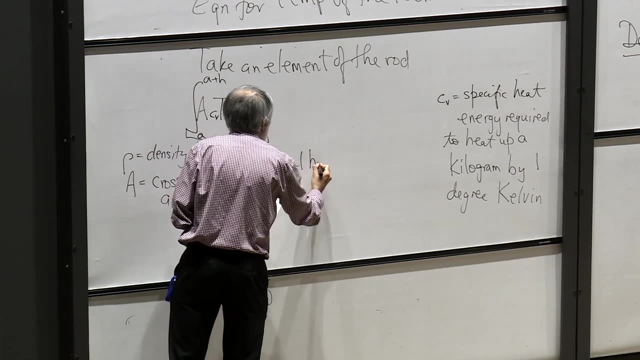 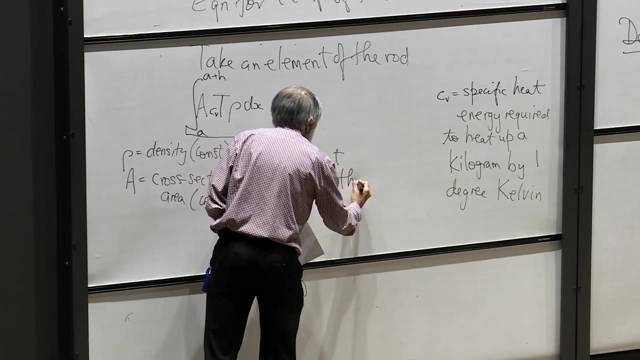 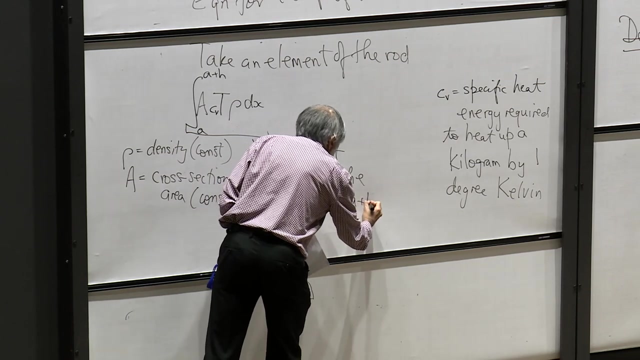 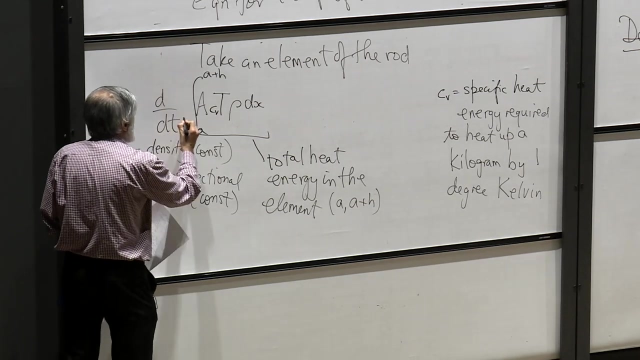 from A to A plus H and that's the total heat energy. Total heat energy, Total heat energy. So the total heat energy is equal to the total heat energy in the element A, A plus H. And now we want the rate of change of that energy. 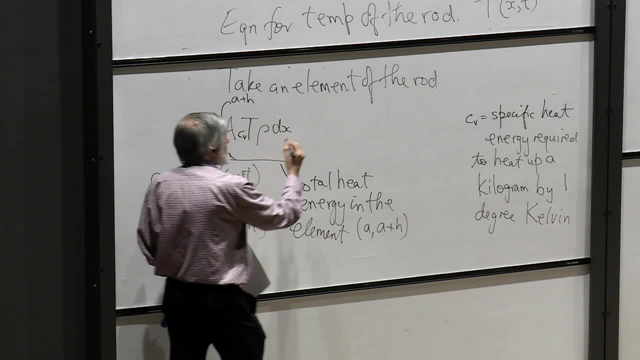 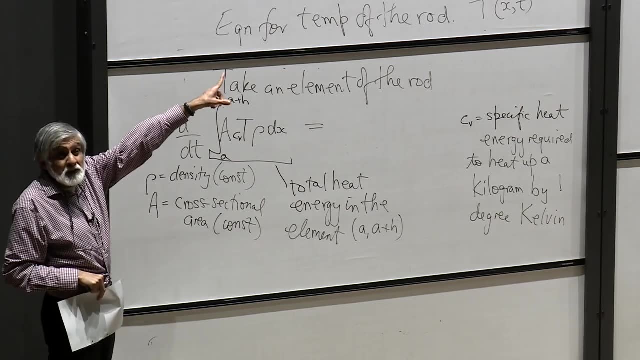 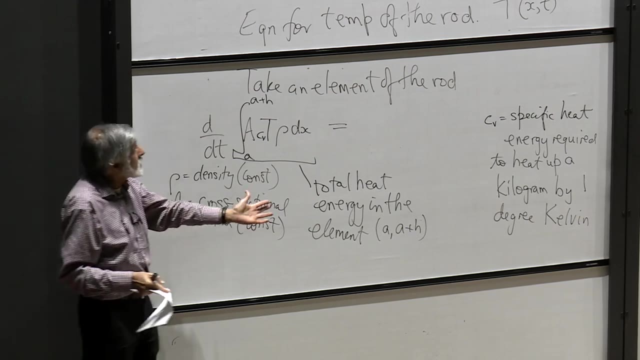 Okay, So how could that energy change? Well, it could, because, be that there's some heating element in there that's producing heat, could be a source of heat, or it could be, and indeed it could be, that heat is flowing. 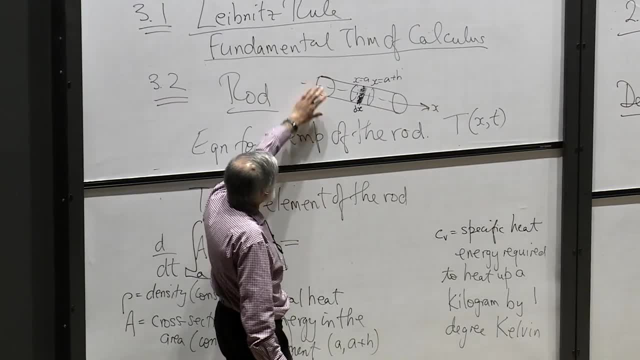 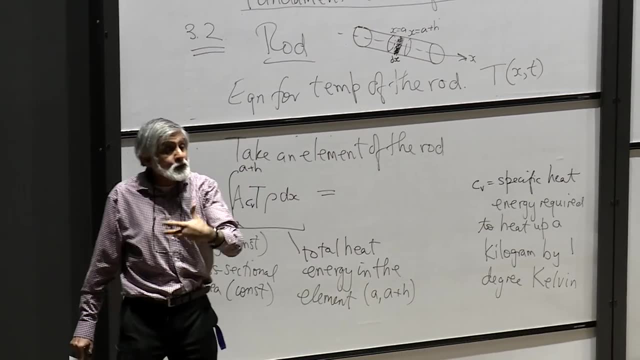 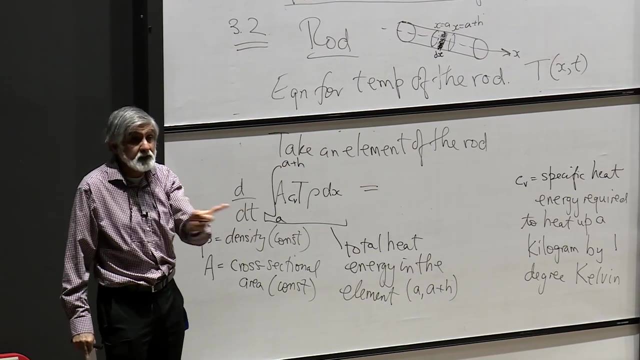 Because maybe you started off by making this very hot, so heat is flowing. So we're going to do, to begin with, assume that there's no source, so the only way the heat is changing is due to the movement of the heat. Okay, So that means 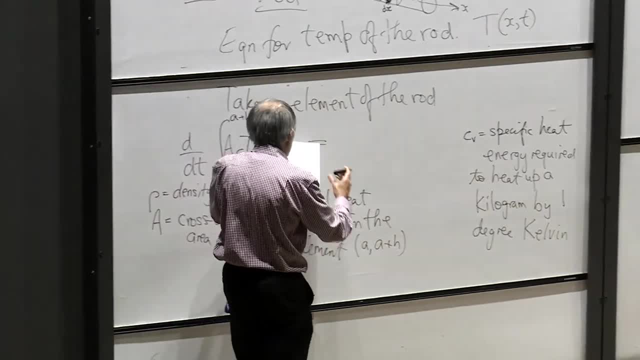 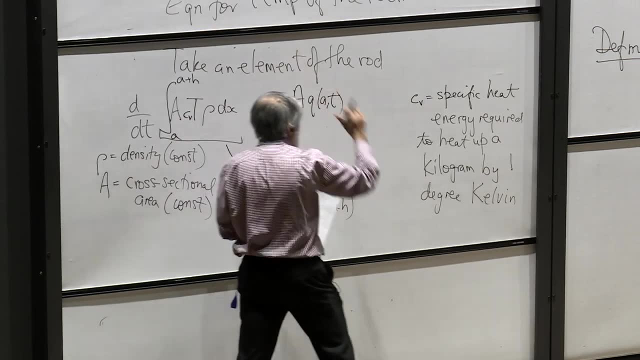 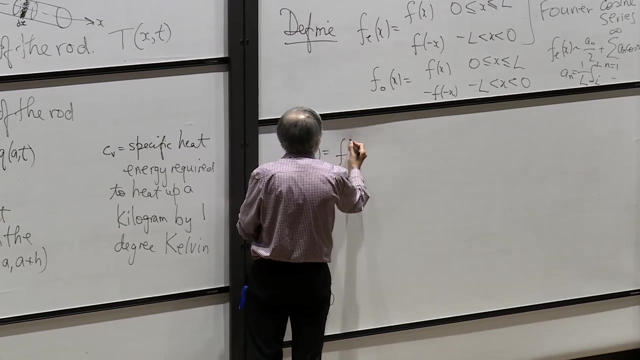 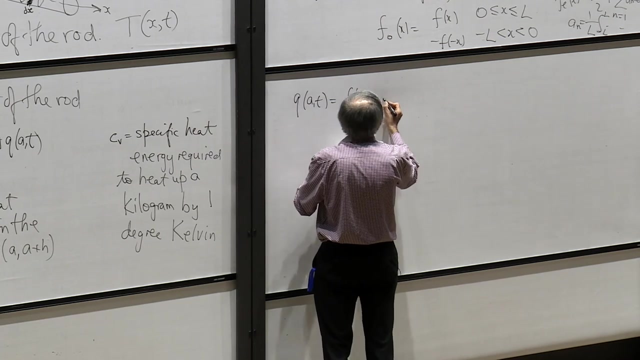 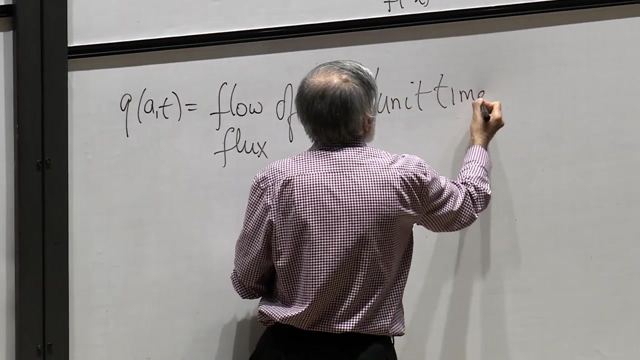 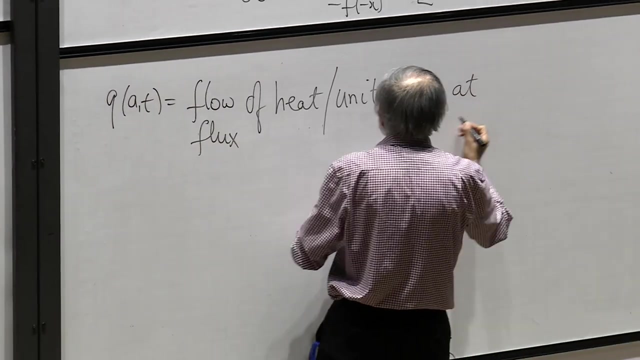 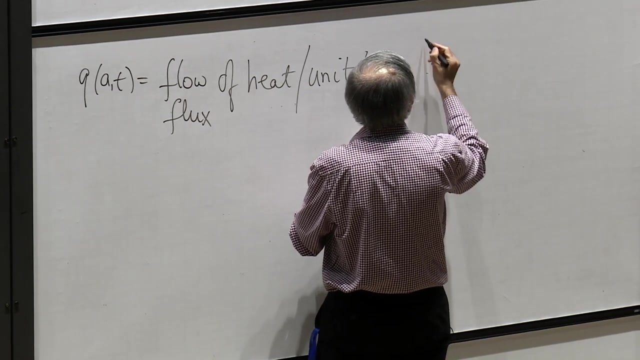 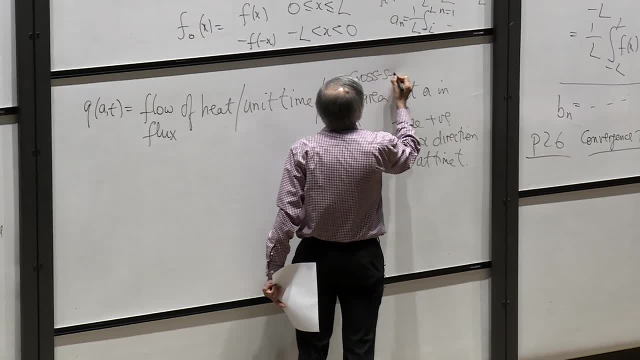 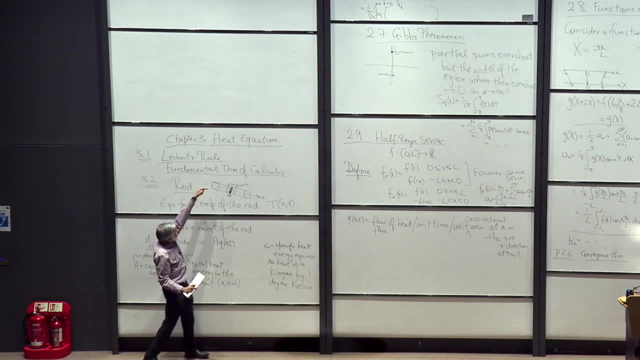 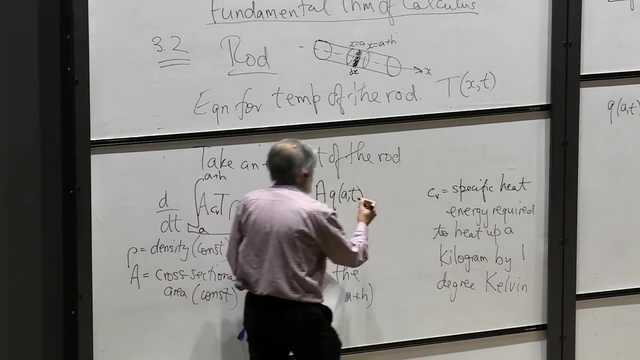 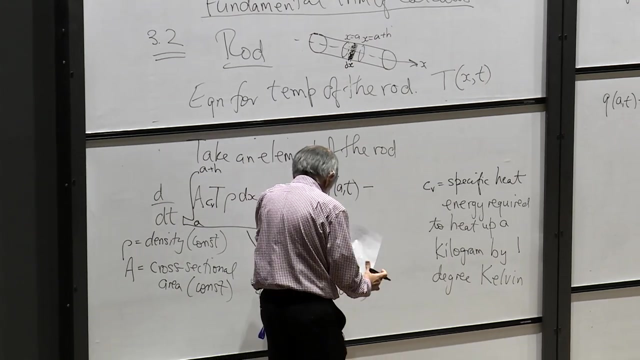 2.4.9, in here. So that will be the flow in. so that's going to increase. so that's a plus there. But then there's going to be a flow out At this point. So you're going to have minus a. 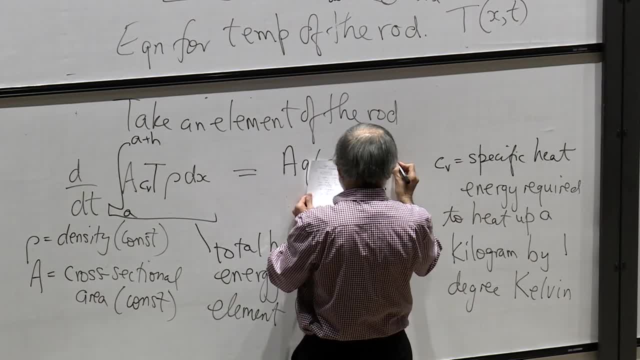 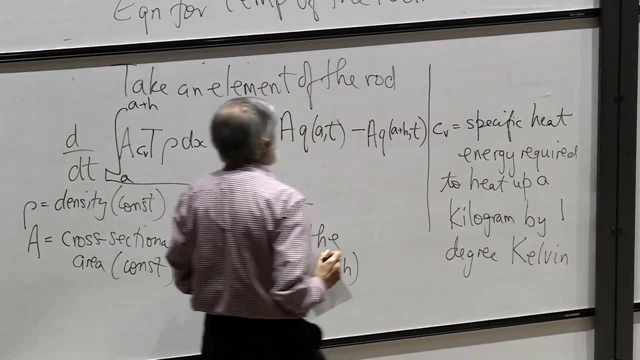 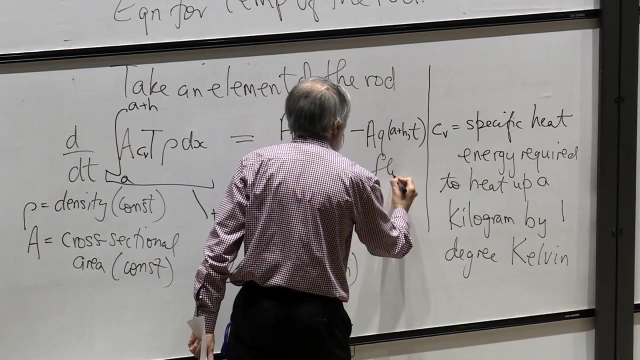 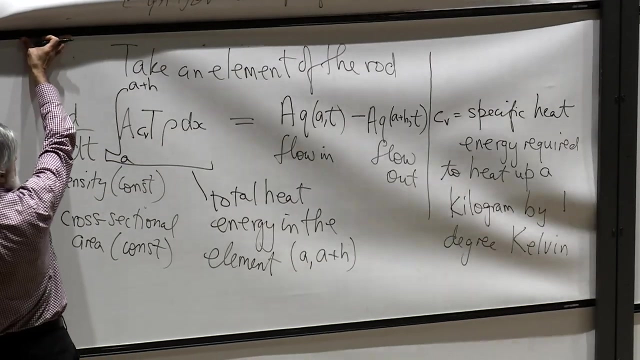 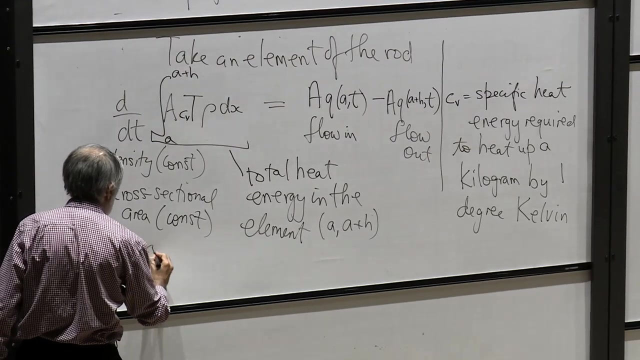 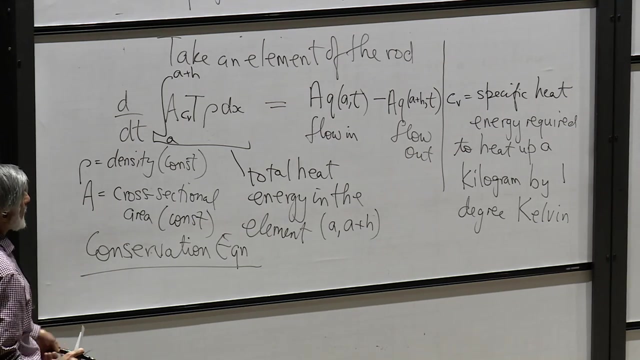 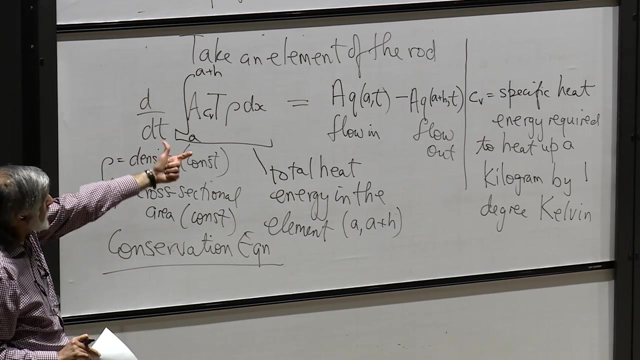 Q of A plus H, T. Okay. so this is flow in, flow out. So that's a conservation equation. Conservation Okay, because the heat doesn't get lost anywhere. so heat going in minus heat going out, that contributes to the rate. 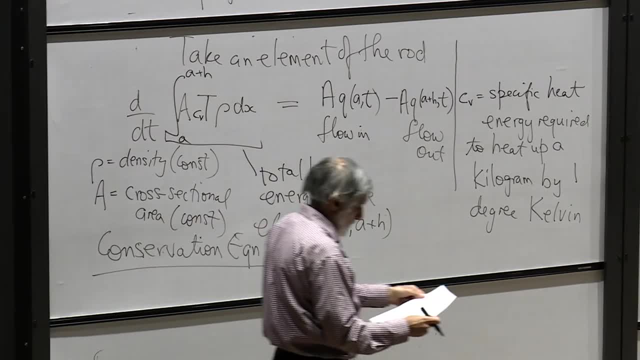 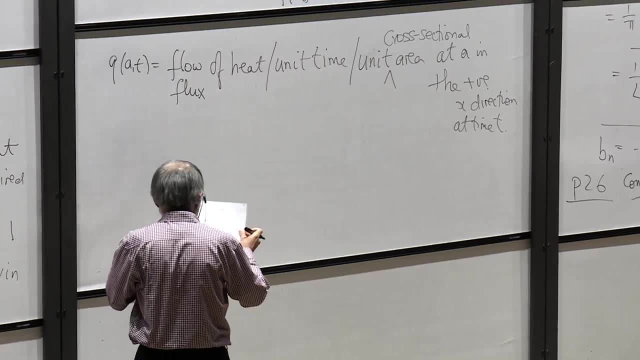 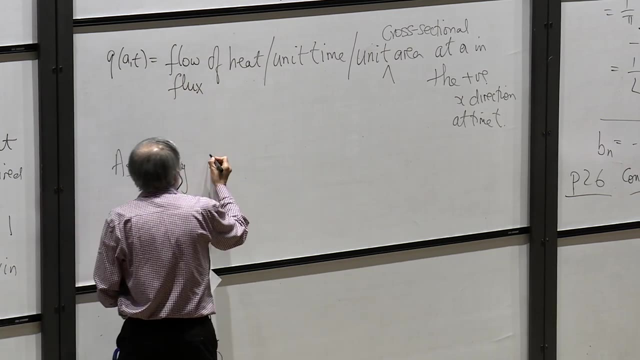 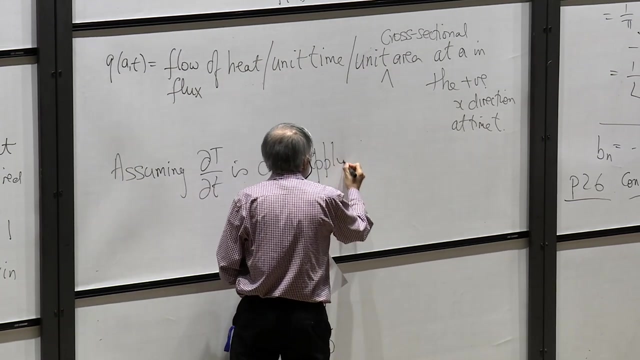 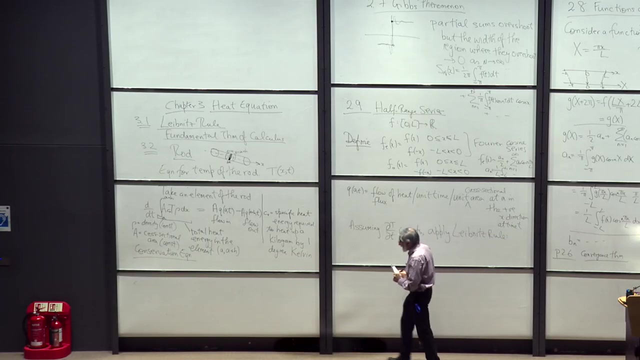 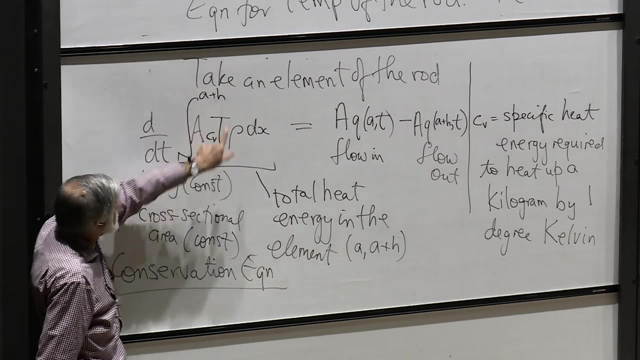 of change of heat. So, assuming DT by DT is continuous, we can apply the Leibniz rule And remember what Leibniz rule said was that if these do not depend on time, then you can just swap these around. but this becomes 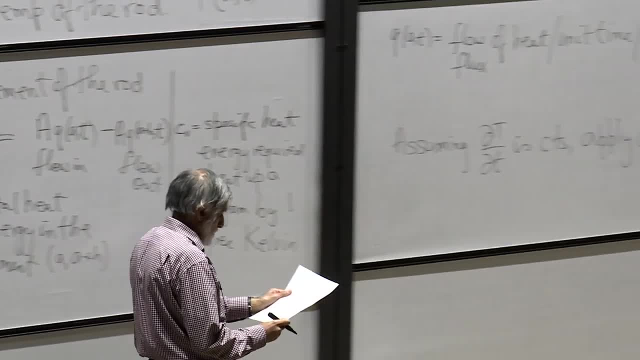 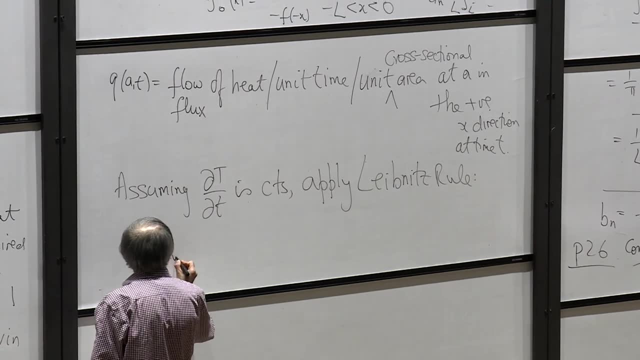 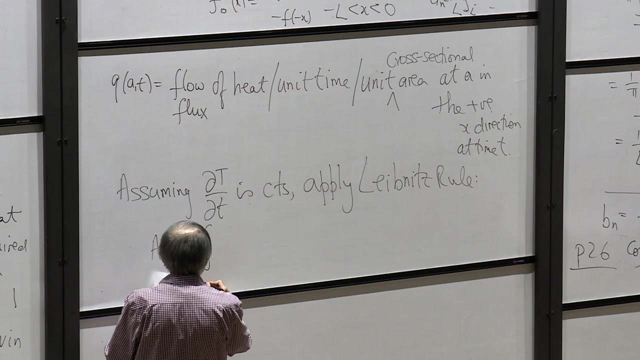 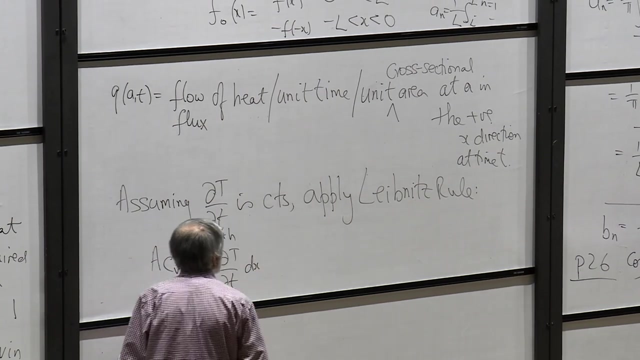 a partial derivative. Okay, So what we're going to have then? and A is constant, CV is constant, rho is constant. that's our assumptions, integral from A to A plus H, DT by DT, DX. and now let's bring these over to this. 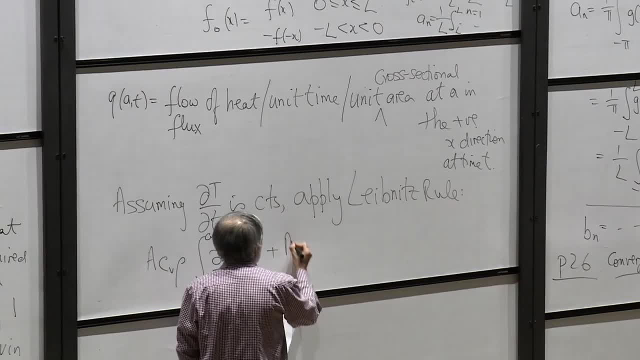 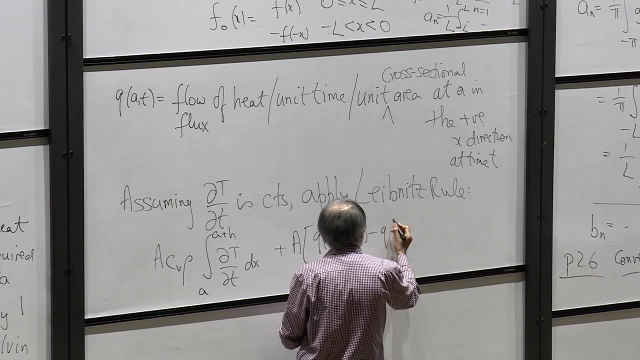 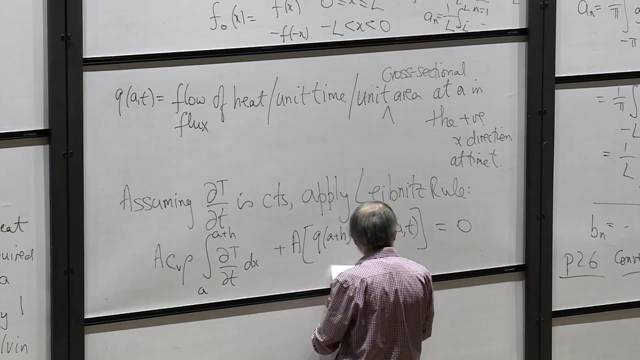 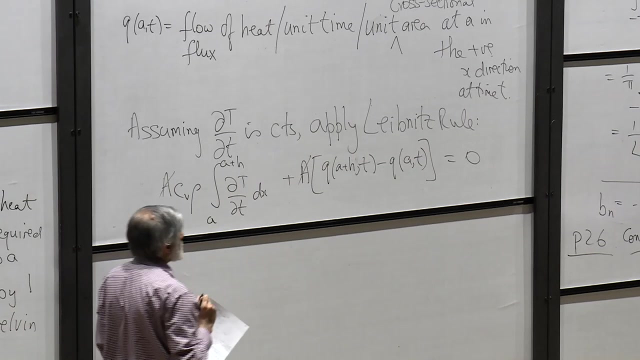 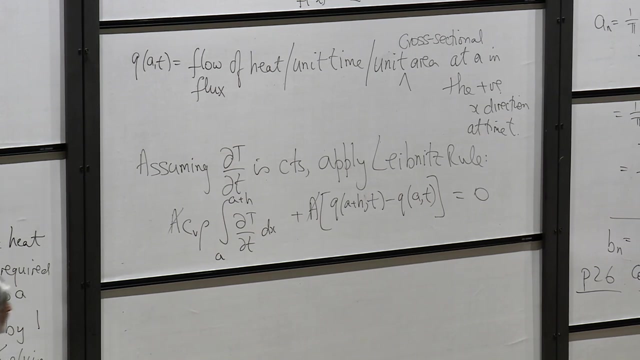 side Plus A into QA, plus H of T, minus QAT equals zero. Okay, And the A's cancel. And then if we look at that, we can see that we sort of say: look at this thing here, this reminds us of a derivative. 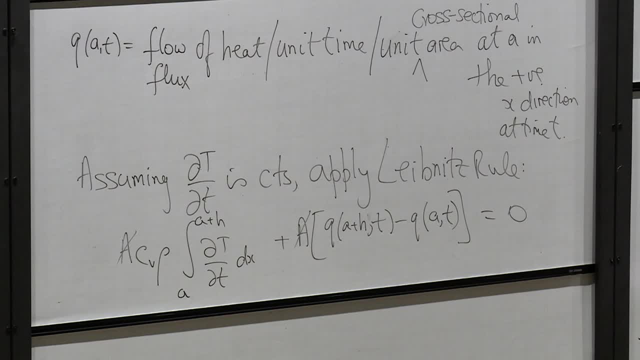 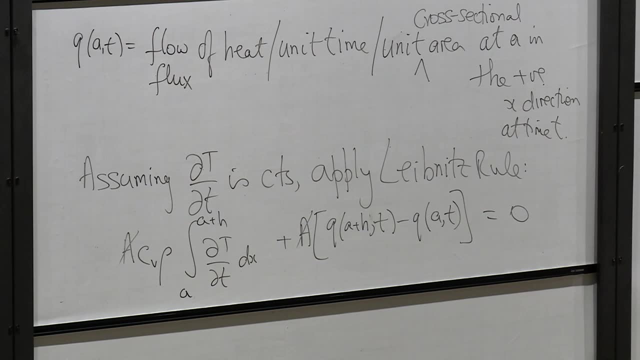 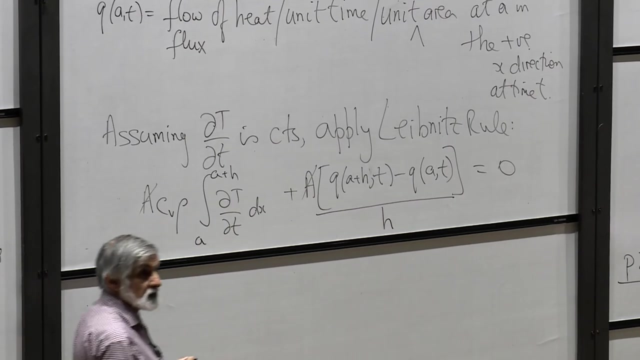 But the derivative would have an H on the bottom line And that doesn't have an H on the bottom line. Well, we can fix that, Just do that. Well, obviously, we can't just do that, We have to do it here. 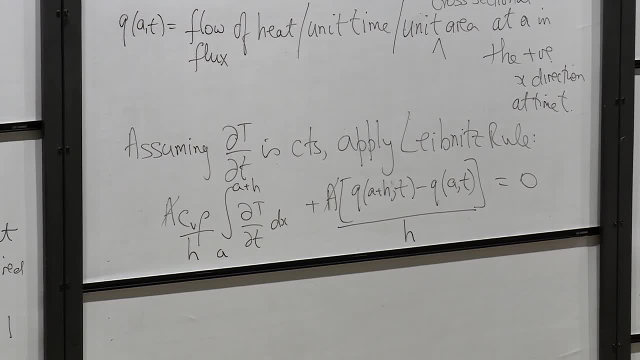 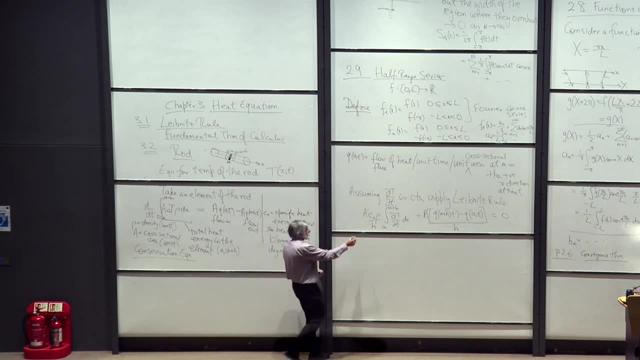 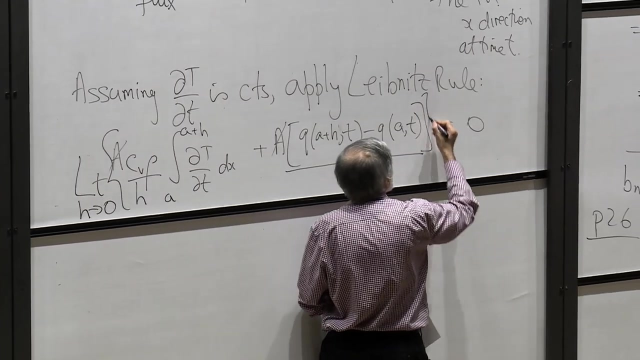 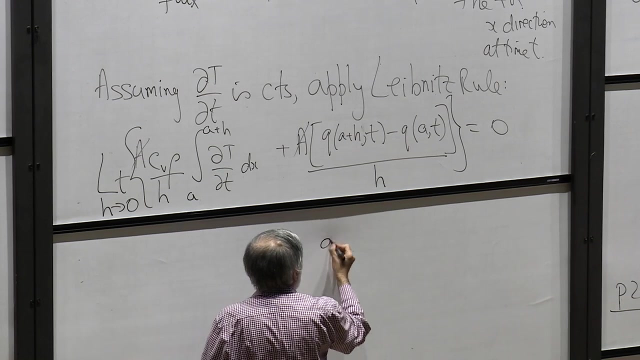 Okay Now, furthermore, the derivative is the limit, as H goes to zero. So why have we done that? Well, this now just becomes dQ by dx, So this is going to be dQ by dx. So this is going to be dQ by dx. 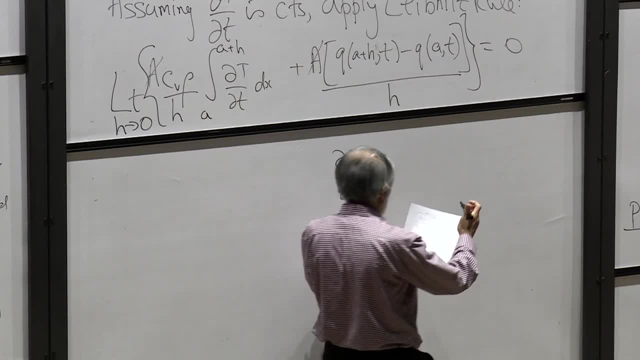 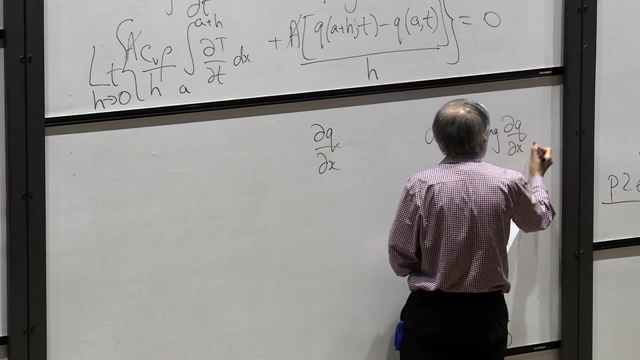 So this is going to be dQ by dx, Assuming that Q, Assuming that Q, Assuming that Q, dQ by dx is continuous, etc. dQ by dx is continuous, etc. And then what does this become? And then what does this become? 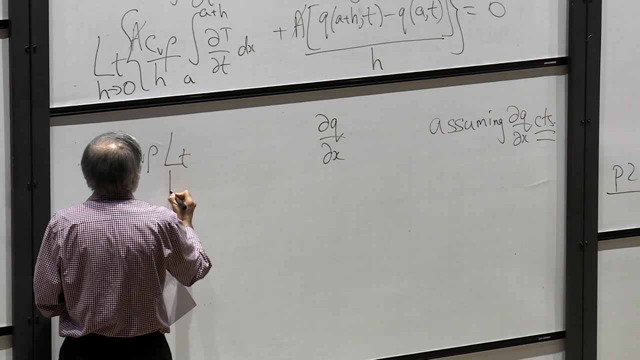 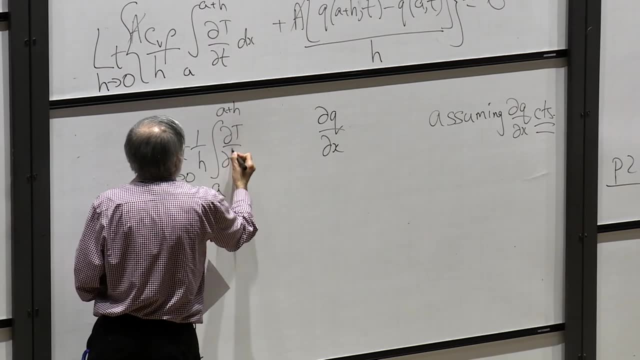 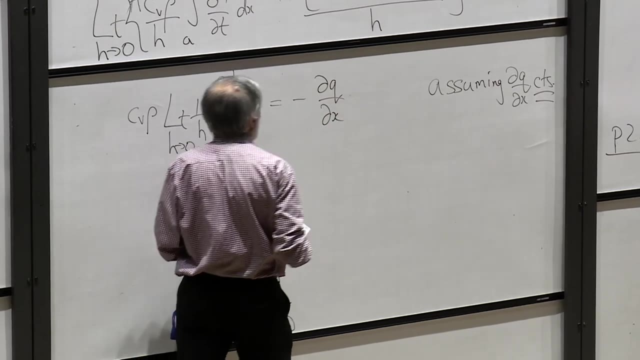 Well, Cv rho, the limit as H goes to zero, the limit as H goes to zero, one over H a to A plus H, dt by dt dx, dt by dt dx. So what I can do, take that over to the other side. 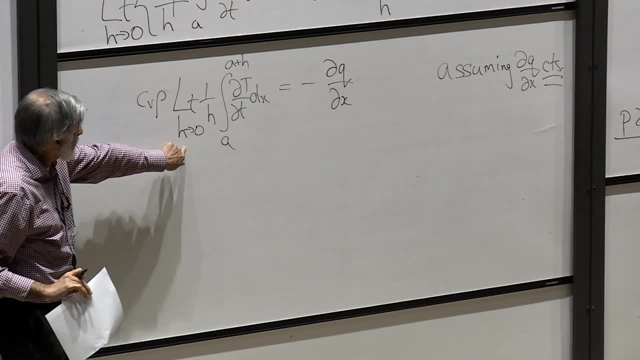 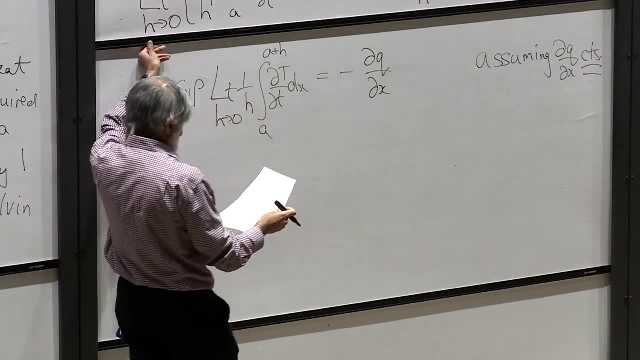 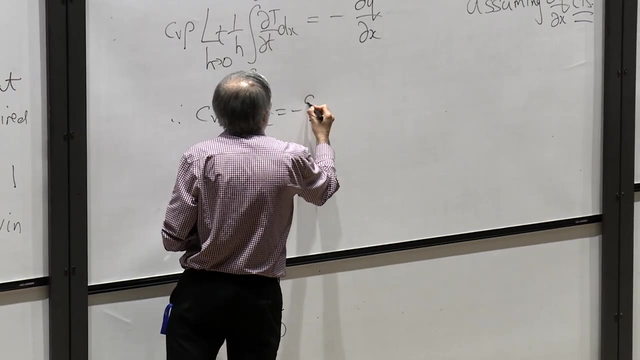 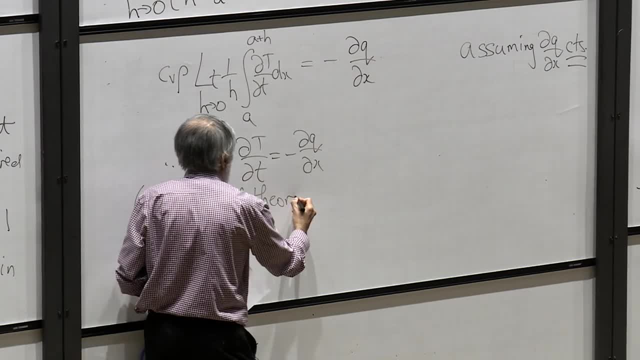 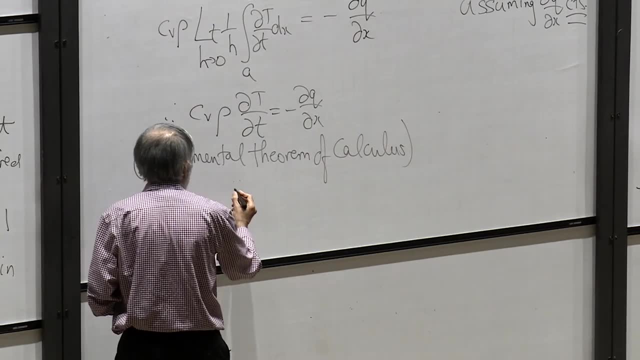 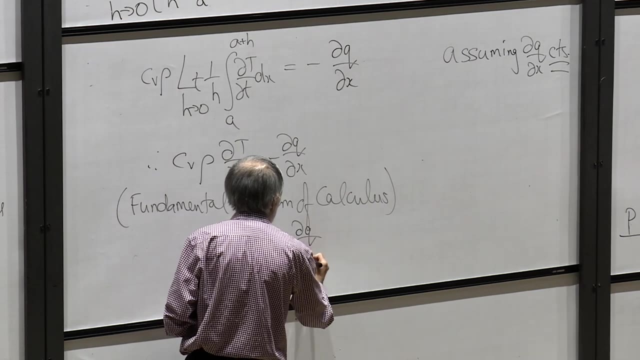 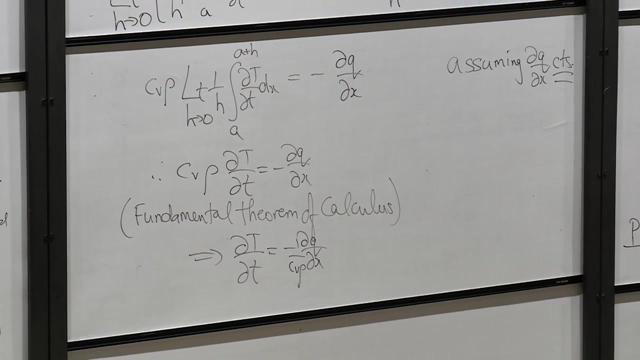 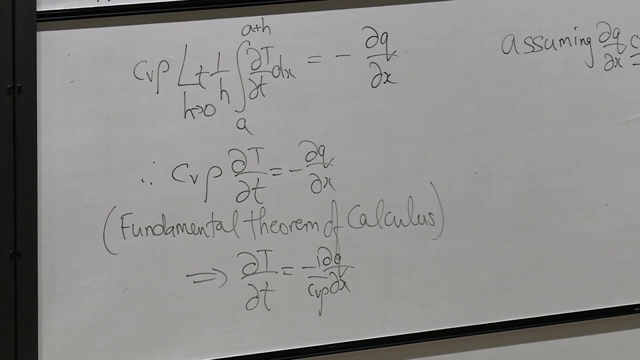 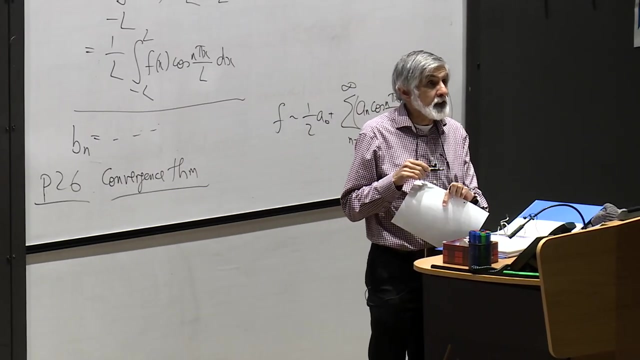 Using the fundamental theorem of calculus. So that gets us that dt by dt is minus dQ by dx, divided by one over Cv rho, one over Cv rho, one over Cv rho. So now the question is: what is Q? So what we've done up until now is: this is all mathematically rigorous, okay. 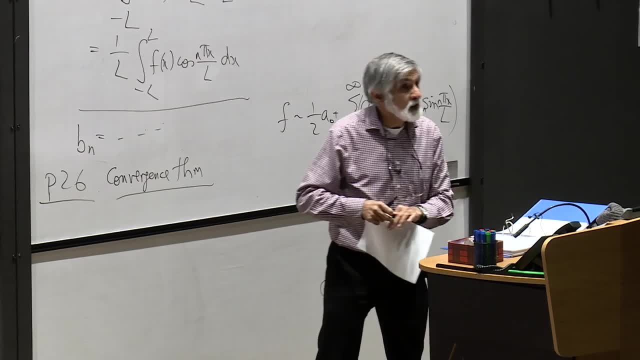 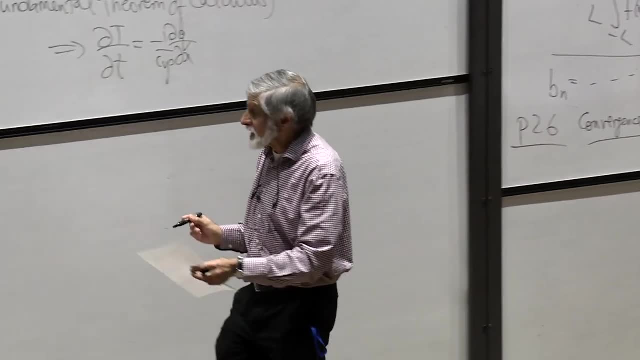 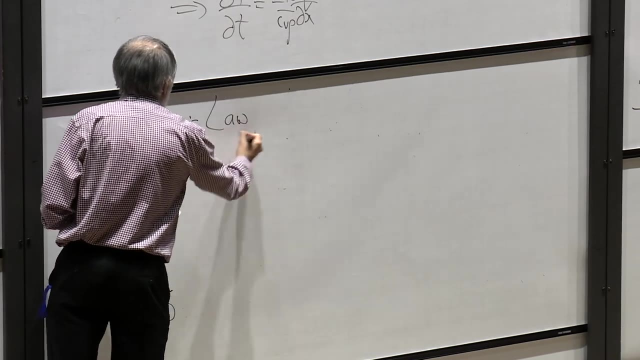 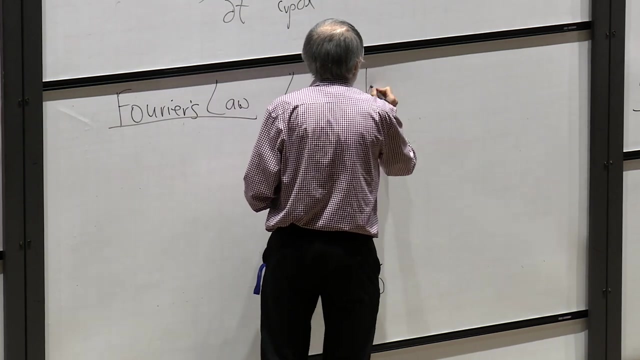 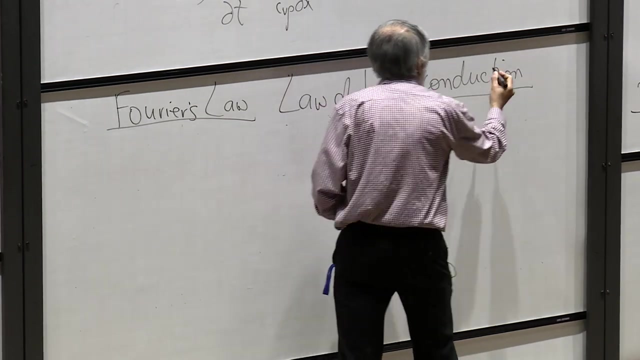 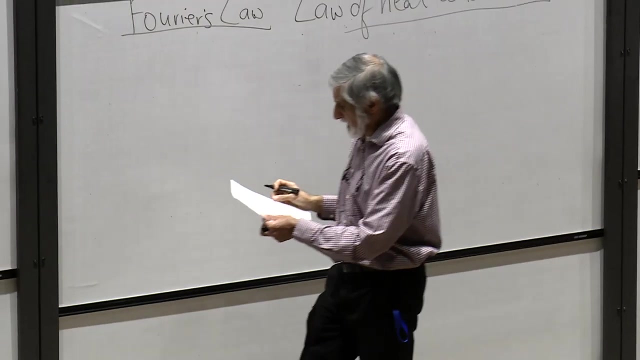 Now we have to do mathematical modeling, We have to make a hypothesis of what is Q And so this is Fourier's law. So Fourier's law states, or the law of heat conduction: heat conduction, heat conduction, the rate. 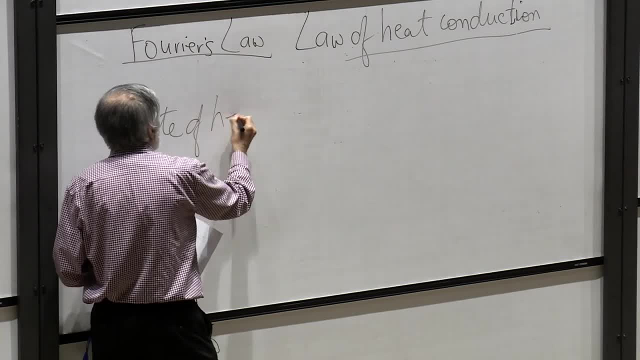 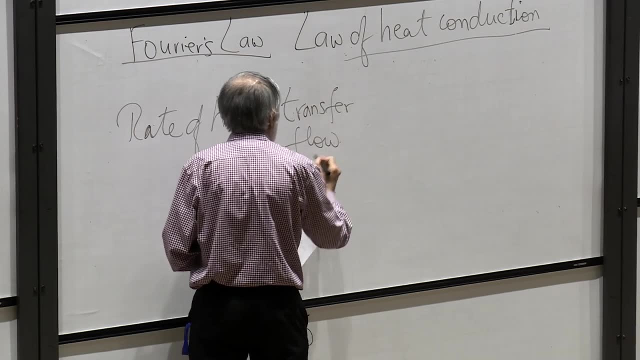 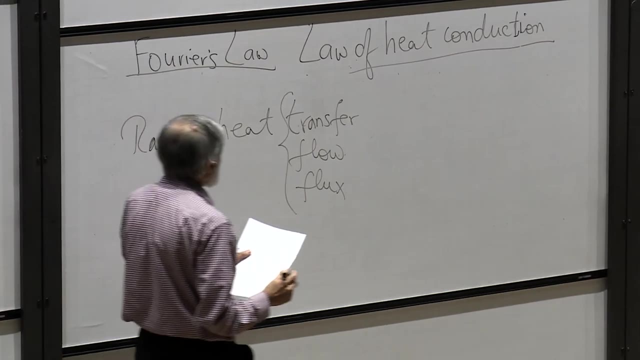 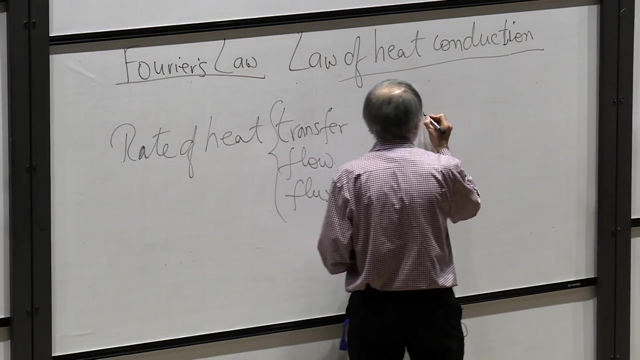 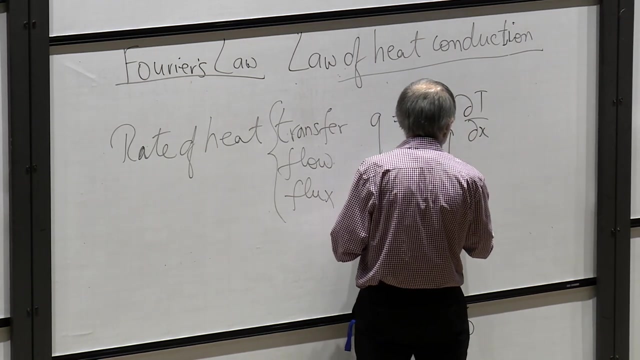 of heat. well, sometimes it's called transfer, sometimes called flow, sometimes called flux. so, all the same, rate of heat transfer: Q is equal to minus k. dt by dx where k is equal to minus k. dt by dx. where k is equal to minus k. 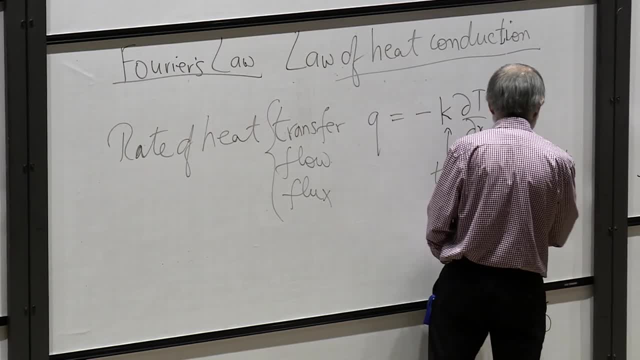 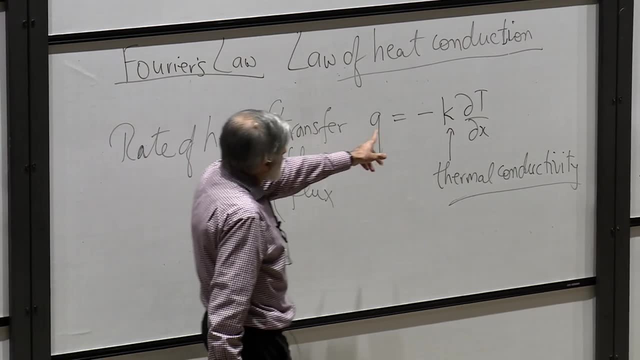 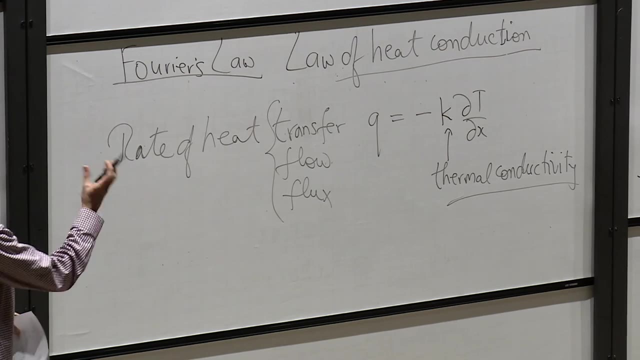 dt by dx where k dt by dx. So all we have to do from that point onward is loop over. J is equal to F, n and Vke to x. We sell thisnek aja j-sink mascot I a-x-self. 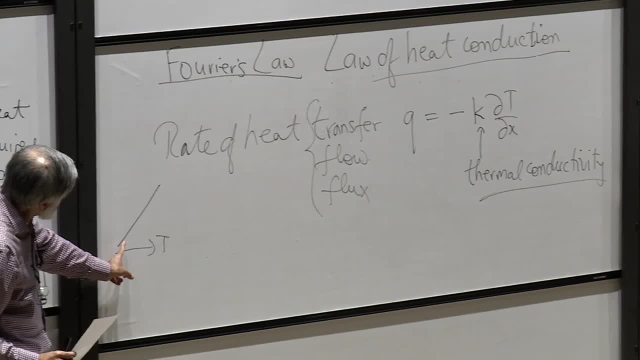 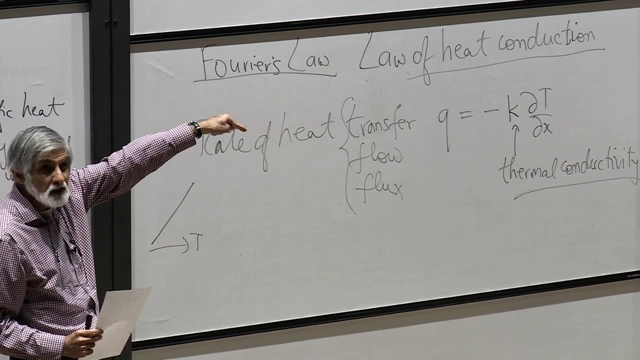 I want to be awesome, So that rooting team is free. Guess we're gonna succeed you guys? All right? See, then dt by dx would be positive, and so they're saying here: q is negative. So that means that heat would flow from here to here. 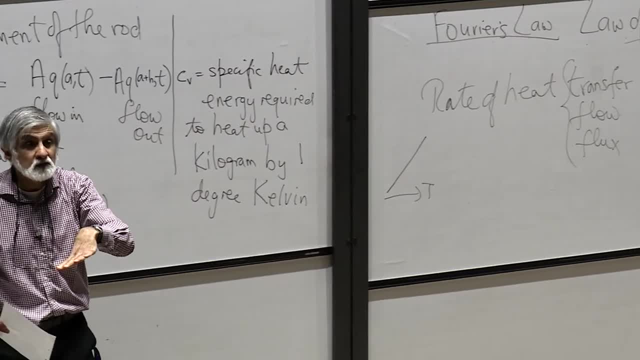 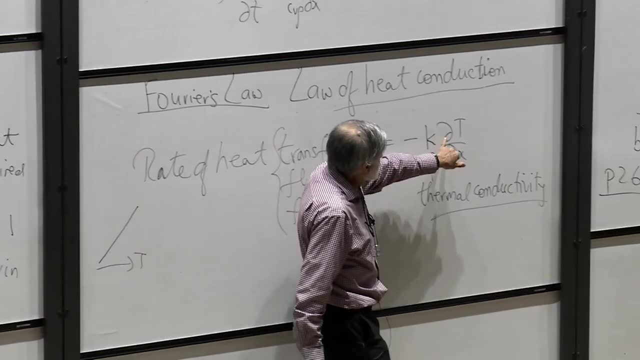 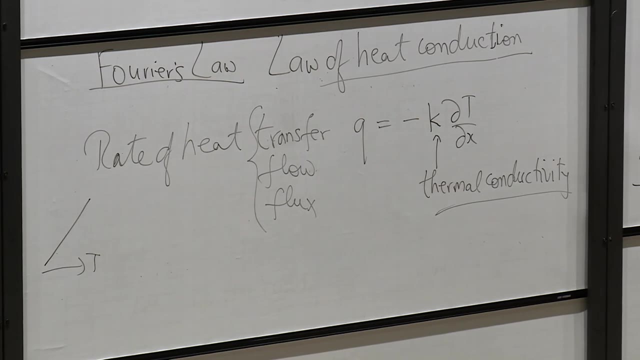 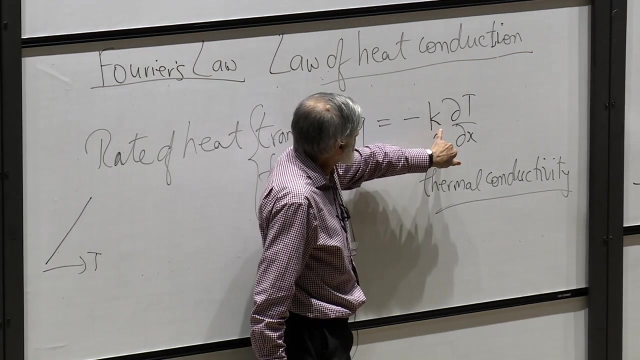 So heat flows from high to low, which seems reasonable. So that's what that's saying, is heat flows down temperature gradients, flows from high values of temperature to low values Seems sensible And it's proportional to that, and the proportion is k, which is related to the conductivity. 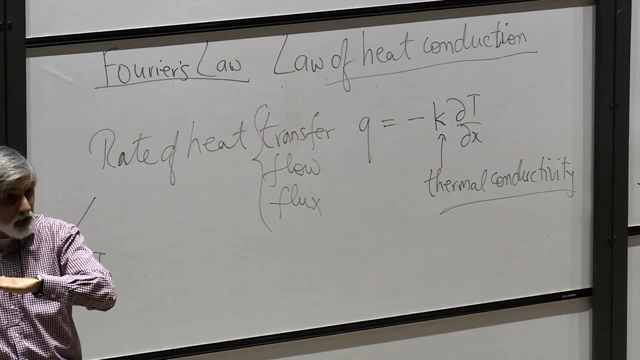 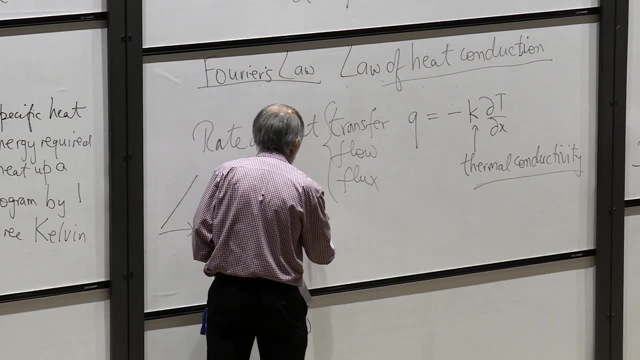 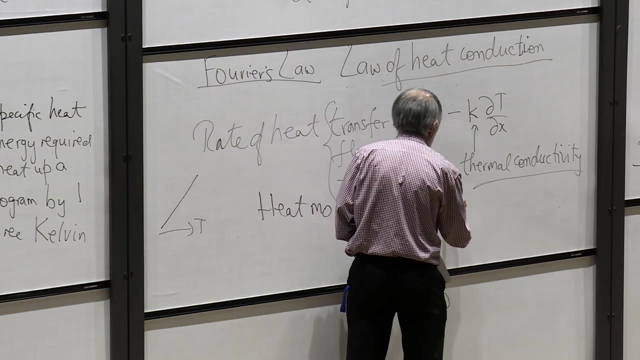 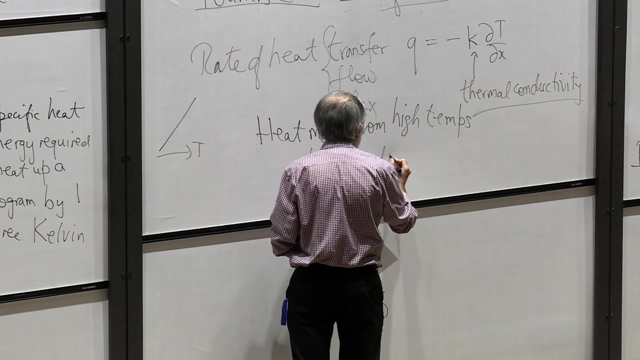 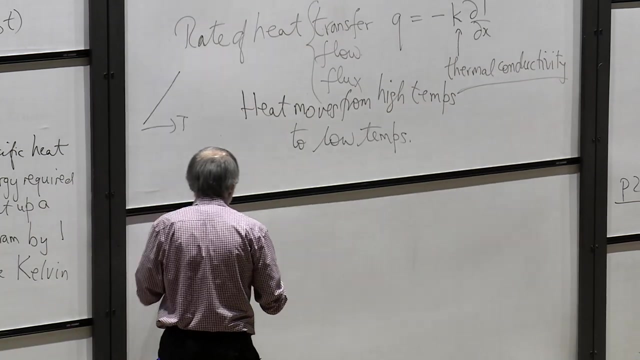 How easy is it for heat to move through the material? So basically what that is saying is heat moves from high temperatures to low temperatures, which seems a sensible thing to do to have as a model. So that means that our equation becomes: therefore: we have dt by d little t. 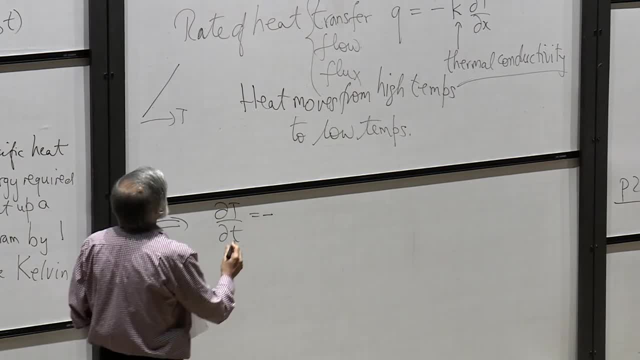 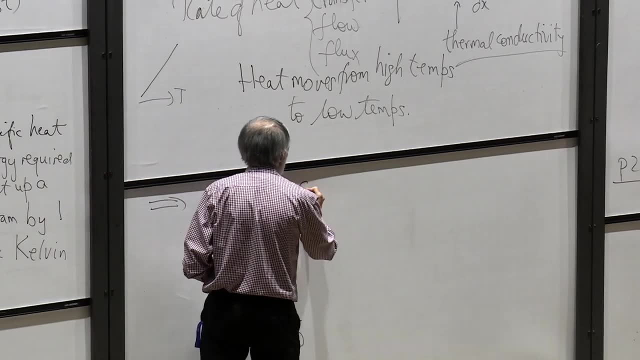 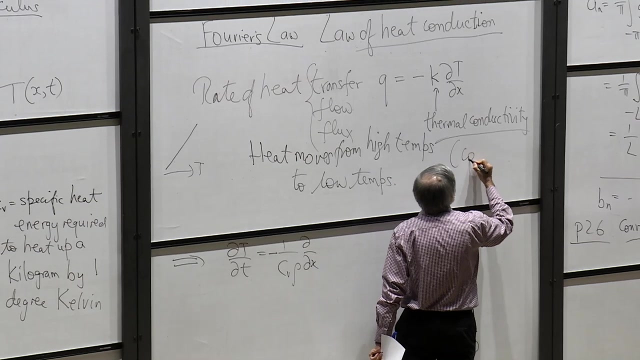 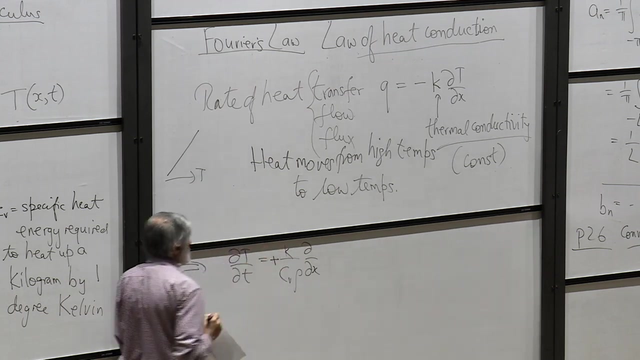 is now minus one over cv, rho, and now d by dx, and assuming that k is constant. and so if k is constant we can take it outside the derivative and that becomes a plus, and then we've got the derivative of t. 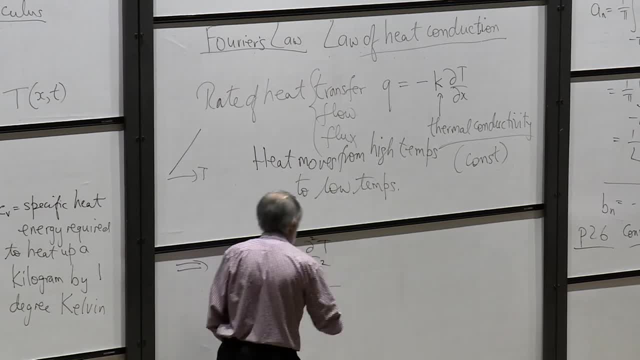 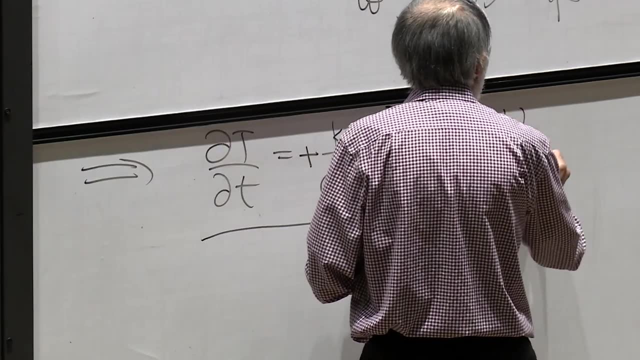 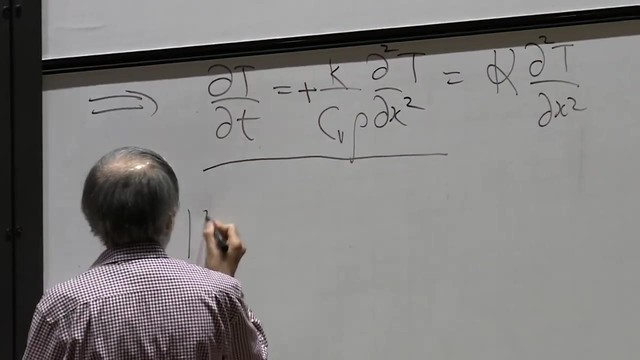 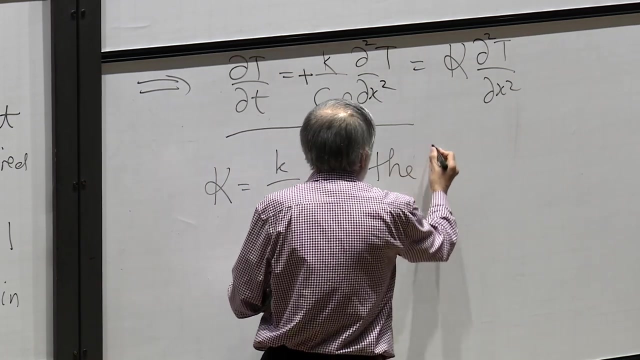 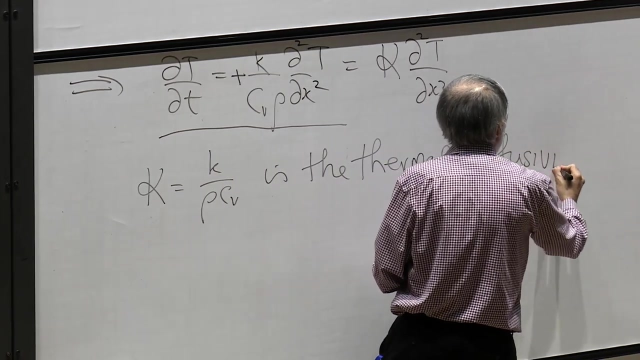 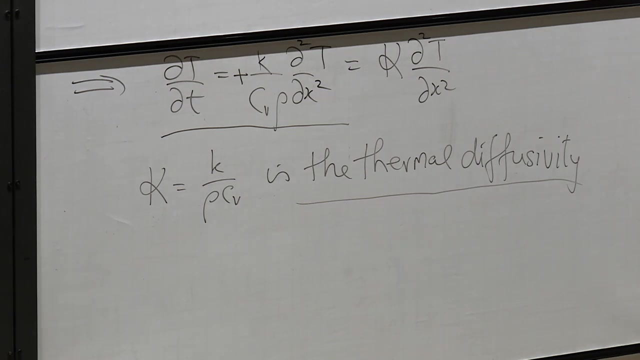 dt by dx squared, And we can write that as kappa d2t by dx squared. where kappa is equal to k over rho, vc is called the thermal diffusivity. Okay, So what this is telling us then? so this is the equation we were solving last week. 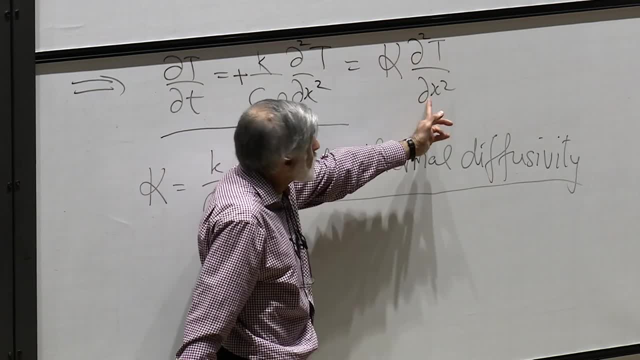 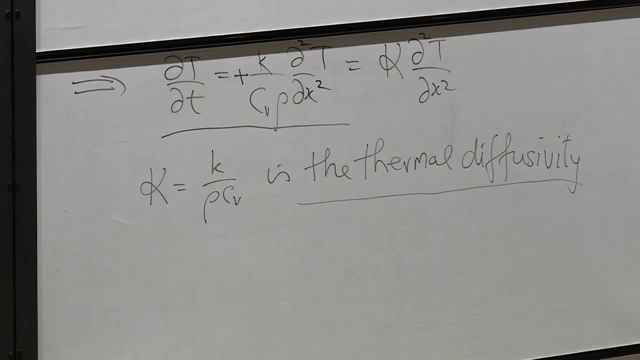 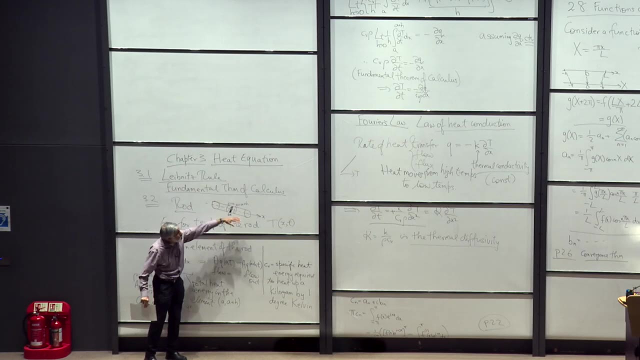 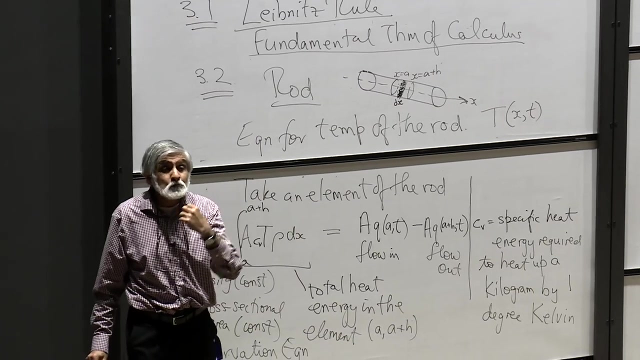 d by dt equals constant times d2t by dx squared. So that's the heat equation Now we talked about. it's called the heat equation because it's movement of heat. Okay, But it could be anything else. It could be molecules of a chemical moving. 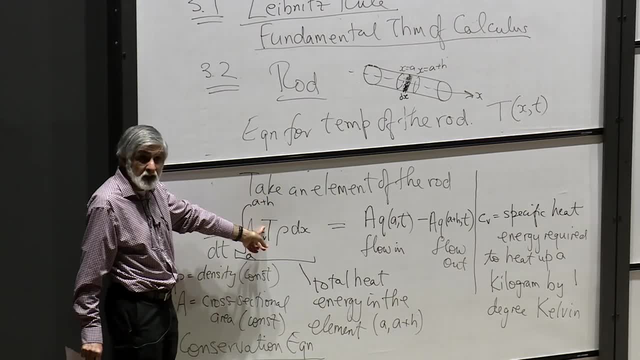 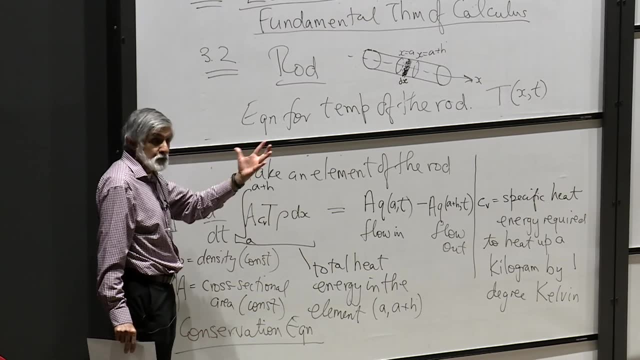 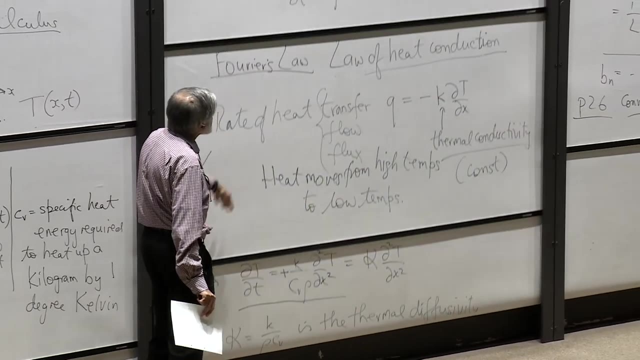 So it doesn't matter what the t is, as long as you multiply by the right parameters here to convert sort of the values in the right way. what you end up getting is this becomes a general formula with some other constants. constant here for the movement of. 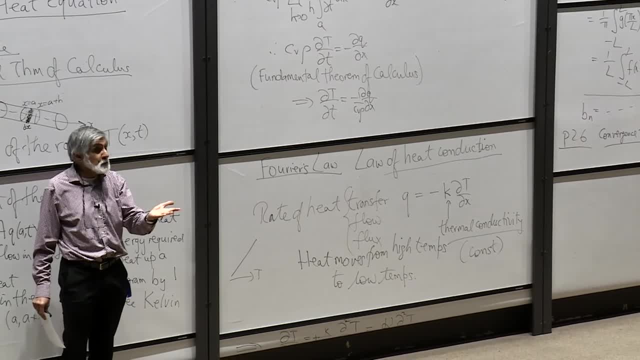 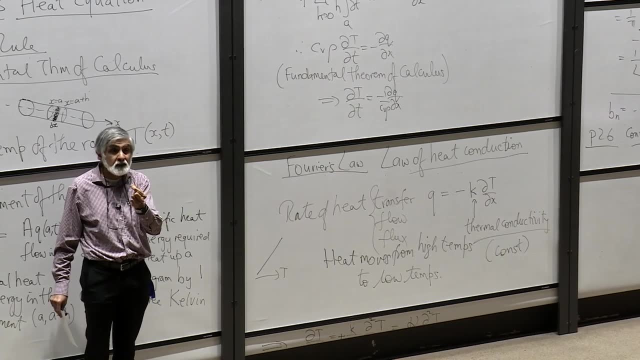 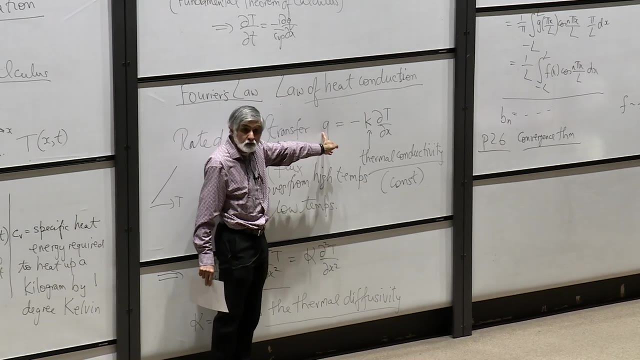 well, he talked about heat, We could be talking about air, We could be talking about a chemical, et cetera, et cetera. And so the key thing then comes in, or we could talk about water. Key then comes in is: how do you find defined q? 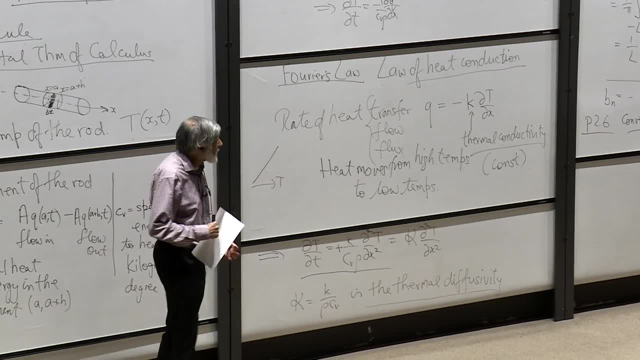 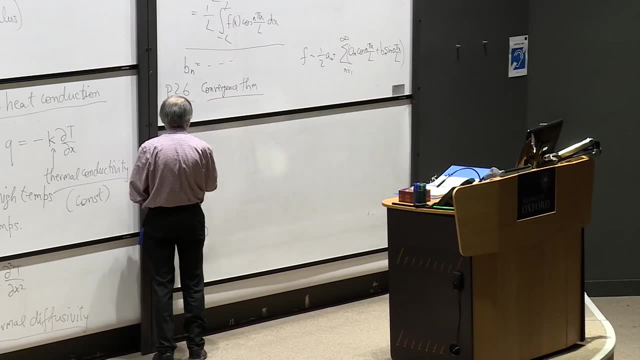 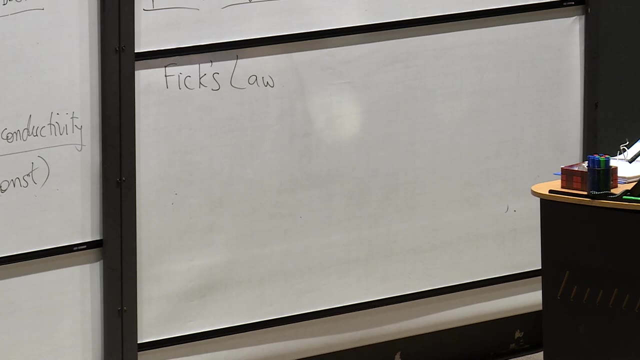 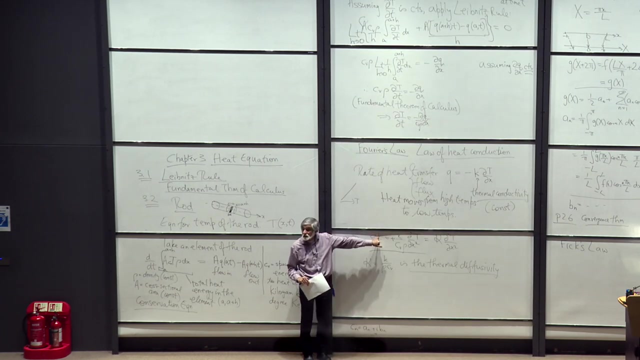 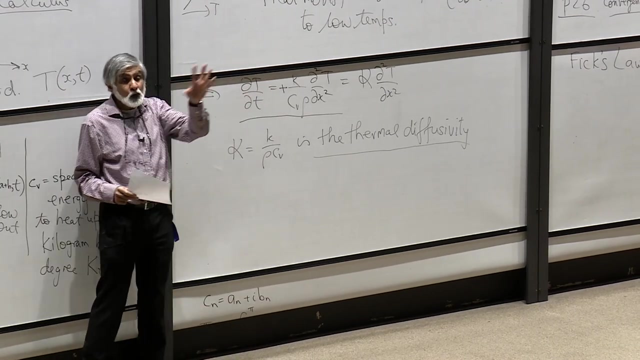 If this is a chemical, you use something called Fick's law. If it's a chemical, it's exactly the same equation, and you get down to this diffusion equation where now this is chemical. Okay, So this can be applied to all sorts of things. 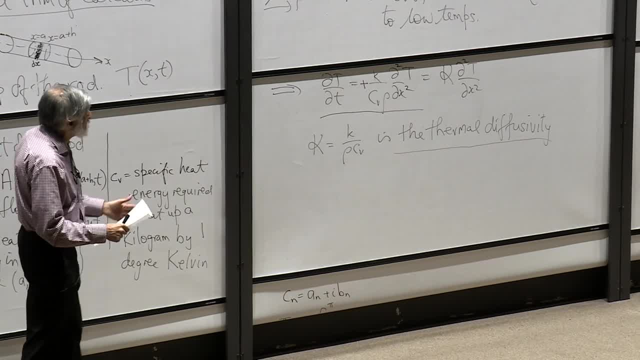 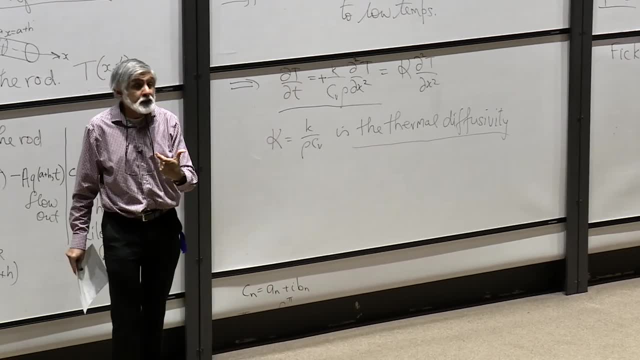 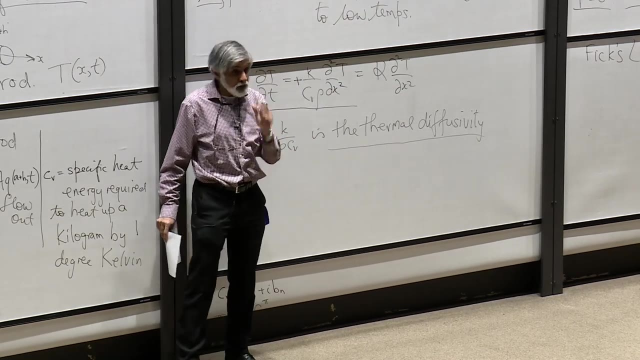 getting this. And so now what we have remember: when we had this equation here, when we tried to solve it, we needed two conditions on x, because we're integrating twice with respect to x and one condition with respect to time. So you could imagine that what that could be. 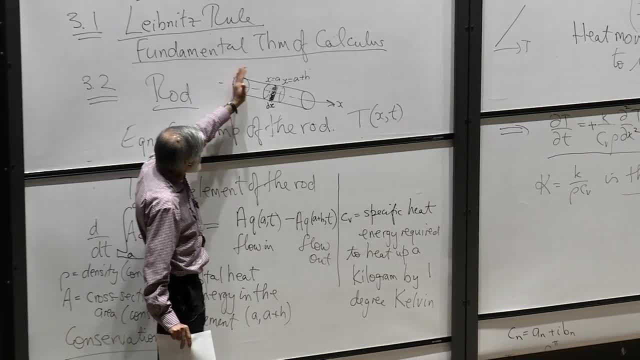 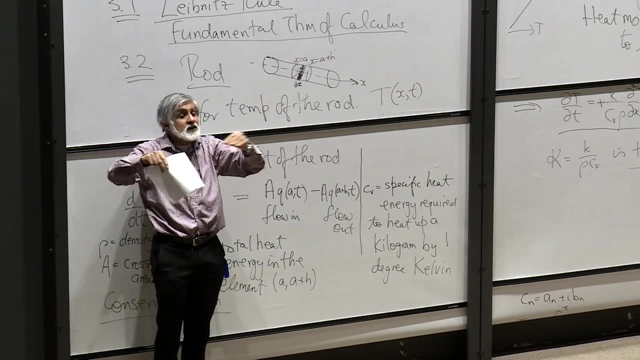 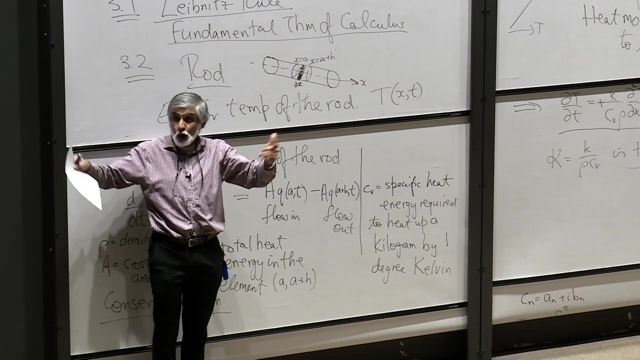 is that we could say at each end of here the temperatures are fixed, Certain values and then initially the rod is of a certain temperature and that's the problem defined. Or we could say heat at one end is coming in at a certain value. 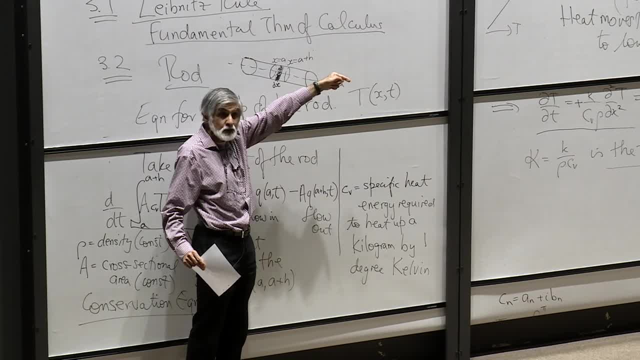 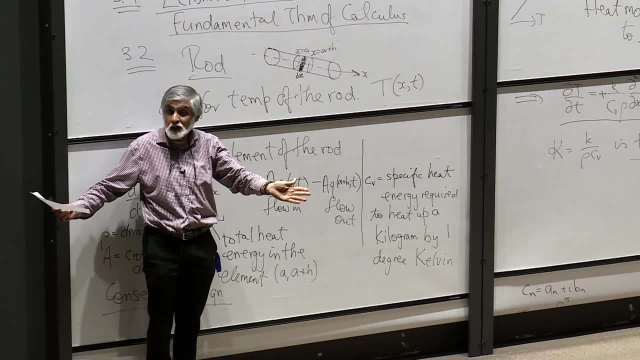 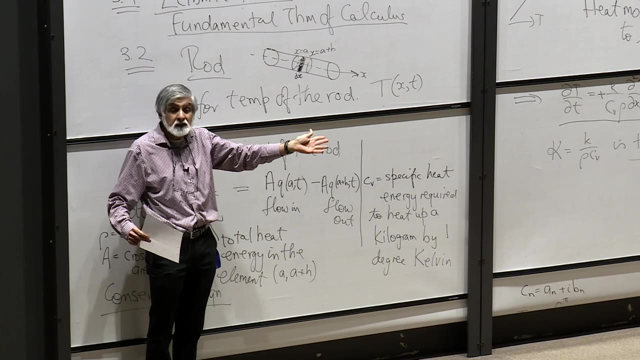 at the other end it's going out at a fixed value and it starts with a certain amount of heat to begin with. There'll be another initial boundary value problem And these are the problems we've been looking at last week. So now you can see the problems that we looked at.